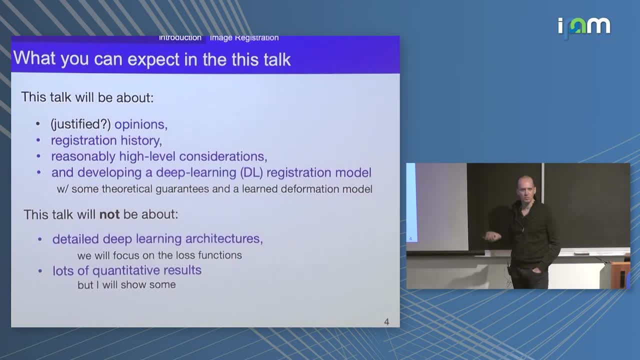 example. So just as a quick overview, what will this talk be about and what will it not be about? So I'll give you a bunch of opinions which may or may not be justified, so feel free to push back. I'll talk a little bit about registration history, sort of like what we used to do, and 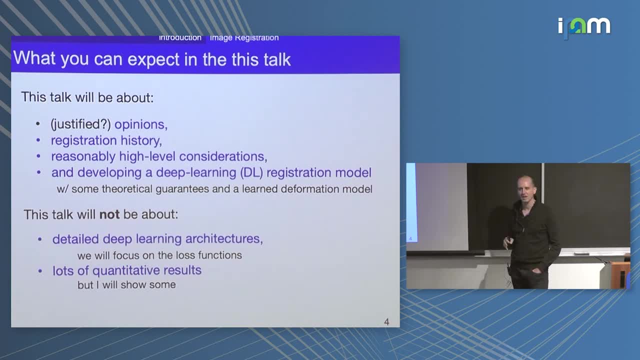 where we're going now. We'll all be at a reasonably high level, but there will be some equations And as we go through this talk I'll try to develop a deep learning registration model. that's sort of a little bit less, a little bit more than these classical approaches in 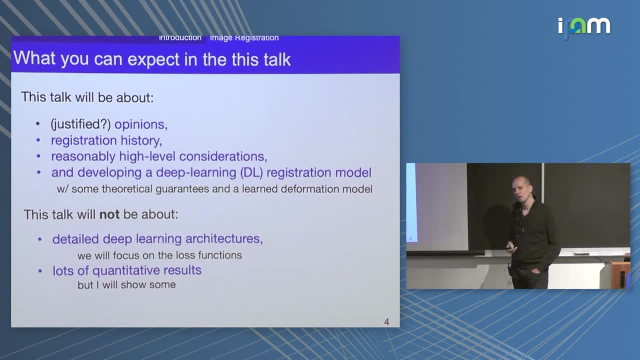 the sense that it has some theoretical guarantees at test time and it also tries to estimate how you should regularize a transformation. So it's trying to push there. I will not talk a whole lot about the data augmentation, but I will talk a little bit about some of the 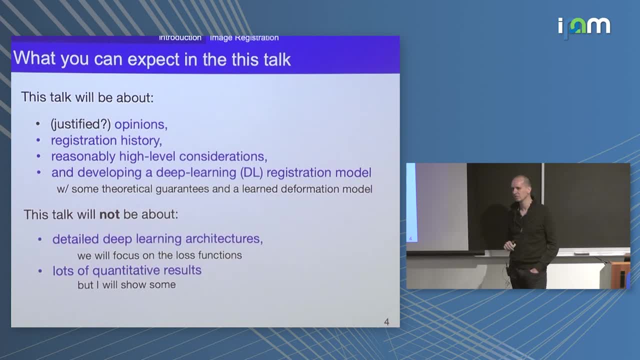 things that I've learned about deep learning architectures. I'll just assume they're given. That's not my focus here, And so I will focus on the loss functions that are used to train these models, And I will also not give you lots of quantitative results. I'll just try. 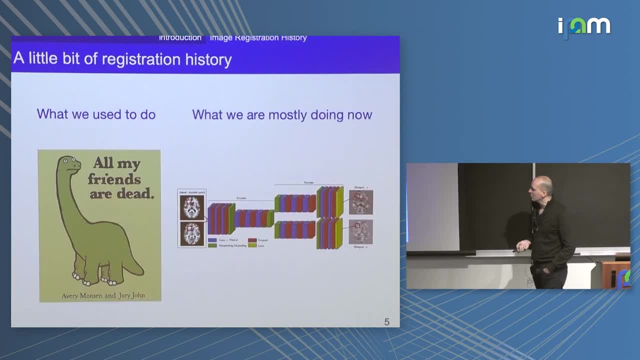 to give you sort of the high-level overview. So what did we used to do? Well, we used to do a lot of stuff just by optimization with pairs of images, and now we push towards these deep learning, registration-based models. So I'll give you a bunch of points of sort of like what classically has been done in. 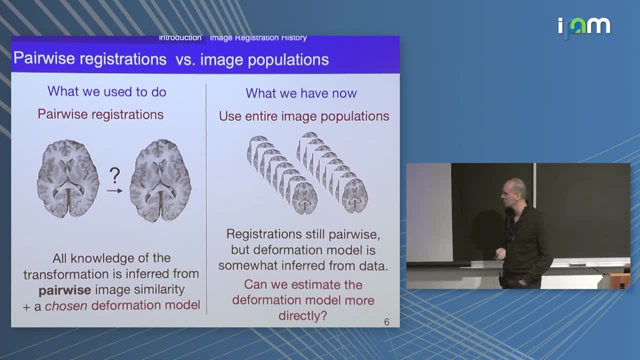 the last couple of decades. So I'll give you a bunch of points of sort of like what classically has been done in the last couple of decades And what has sort of emerged over the last couple of years. So I think the first important. 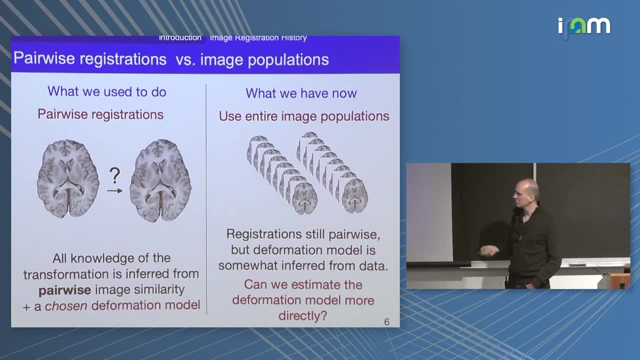 point to make is that it used to be the vast majority of registration methods- maybe with the exception of Atlas Building- was to look at pairwise image registration. So you have pairs of images and that's it. You put your model on it and you do something with this. 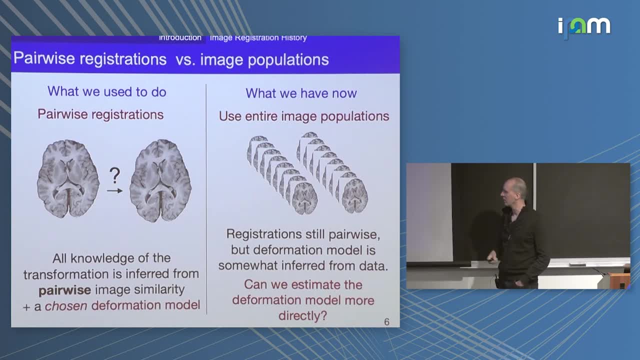 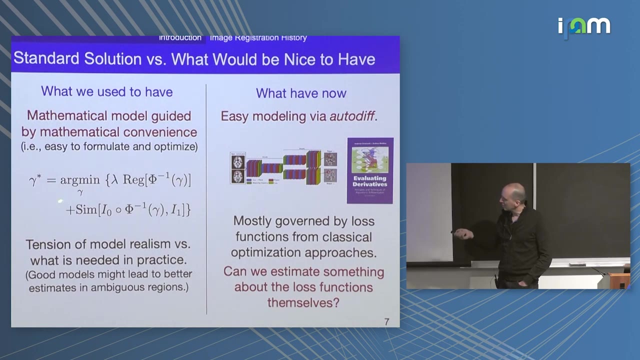 pair of images. Now it's really trying to do something with entire image populations, and this has certain benefits in the sense that you can learn something about the space that these registrations should be living in in the first place. We also used to be guided. we write down mathematical models and often 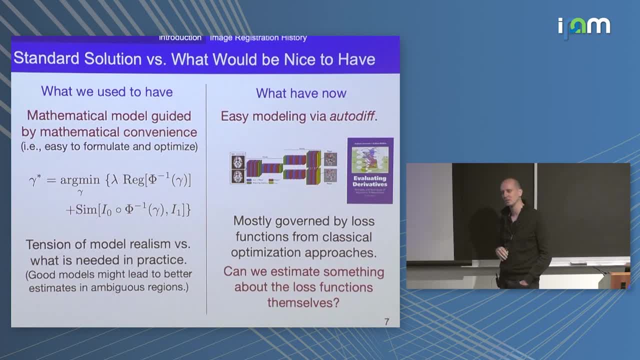 times they were motivated by sort of like a mixture between what you would like to do and what was mathematically convenient in terms of like what you could write down and easily optimize. A lot of these things, I think, have now become much more flexible. 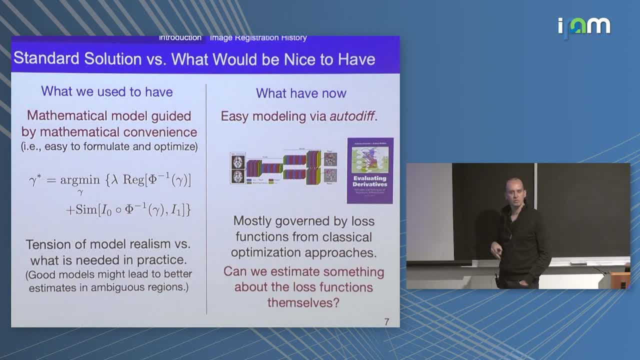 because we can do everything with these deep learning toolboxes. You can use automatic differentiation and you can write down really complicated models. Some of these models, I think, that I'm going to talk about today. sure, you could approach them in the way people used to do them, but I think it would be rather 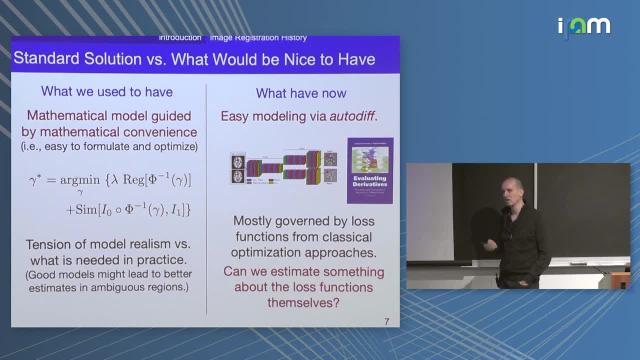 error prone and kind of complicated. So I think, even if you don't do deep learning, if you're in registration, if you use these deep learning toolboxes, I think they're a powerful tool just for very rapid prototyping, because you really can focus on the model. 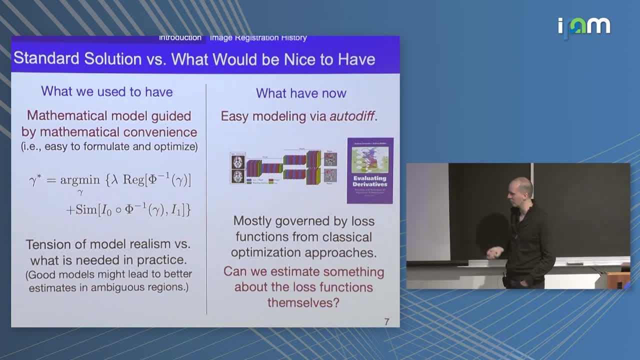 rather than on the nitty gritty behind the scenes details, if you want to play around with them a little bit. Solutions used to be rather slow. You could write down a number of these things. One of the things that I found interesting was that the way a lot 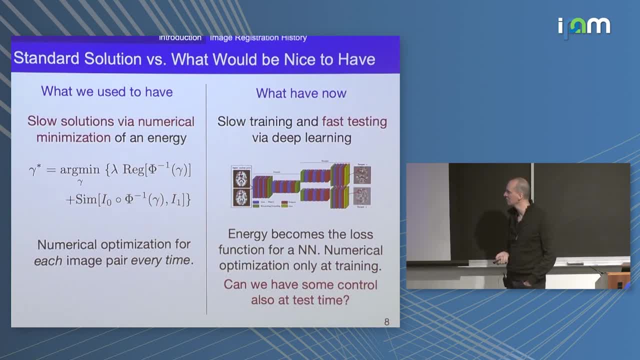 of these things are built is very, very slow, because everything is based on potentially very high-dimensional optimization. And now, when you do this with these deep networks, you get to much faster solutions. Training may be very slow, the training time- but at test time you're just evaluating a regression model, essentially, so you can get blazingly. 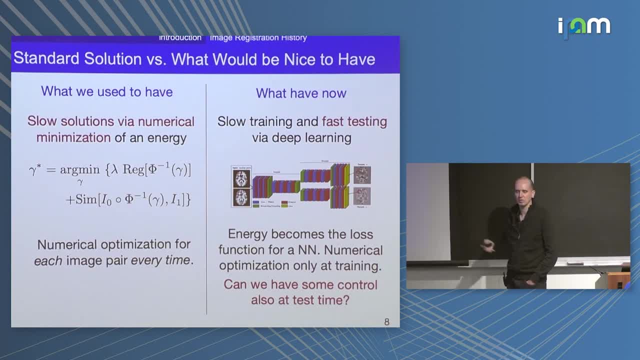 fast registrations And I'll show you some of these results where you can do 3D, 3D volume registrations in a matter of a few seconds if you want to. The question that arises here is that anything you train here on on these loss functions, typically you have control. at training. but even in the case of the cost, you have control on the number of transactions, the number of transactions, the number of times that you have the cost, the cost of the cost, training, because you're minimizing some sort of loss. 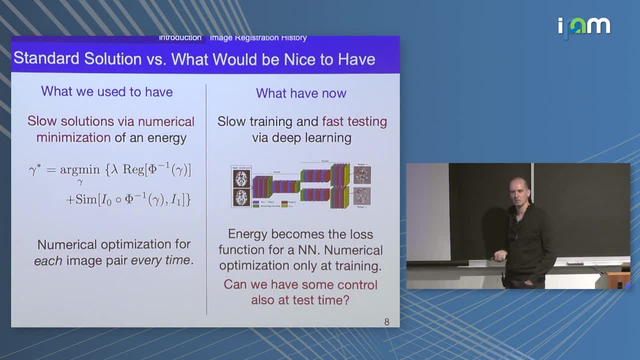 but it's not really clear what the control you have over at test time, right, And if you went to Tom's talk yesterday, it's connects a little bit in the sense when he was talking about like having segmentations and manually correcting them. 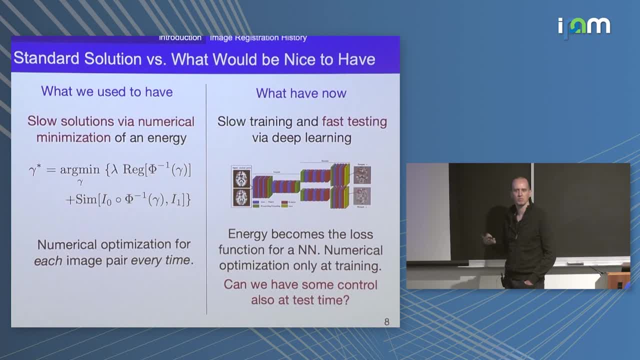 If you do this in a naive way, I mean you can sort of like retrain the network but may not respect what you wanna do. So it's the same kind of setup, right? Maybe you can do something in this registration models. 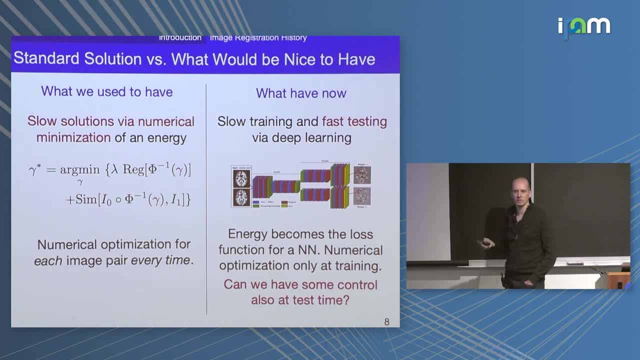 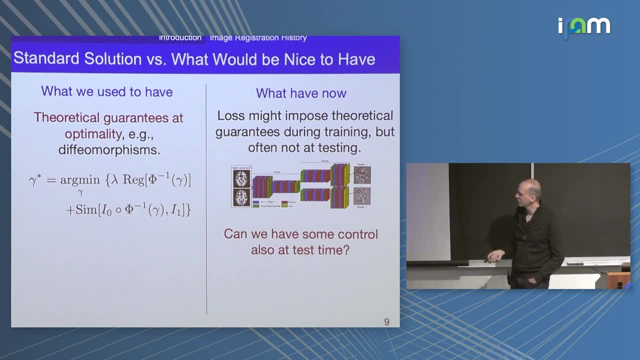 where you try to construct them in such a way that they retain certain properties also at test time and not only during training. Yeah, it sort of goes in the same direction. So, for example, people used to make a pretty big deal out of having diffeomorphic transformations. 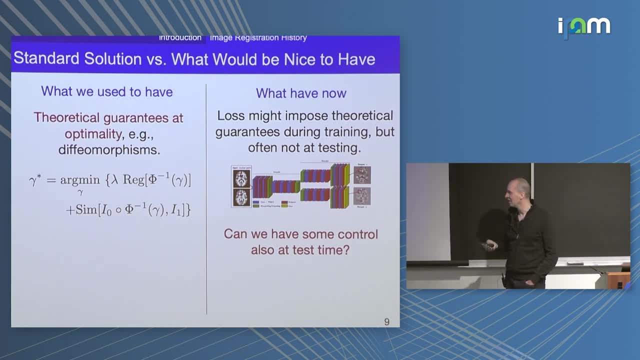 If this is what you want, sometimes it's good, sometimes maybe not. The models that I'm gonna talk about will have this guarantee, but it's the same story, right? I mean, if you do something and you predict something with regression, you may want to have this control. 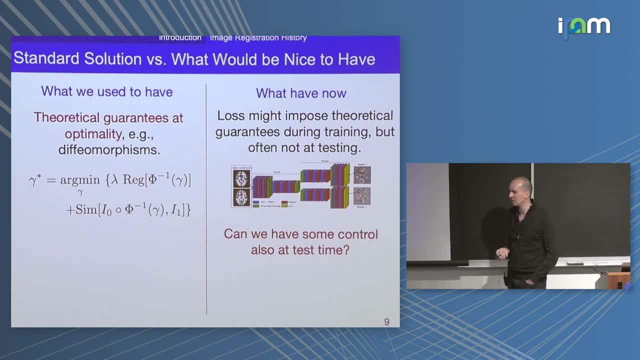 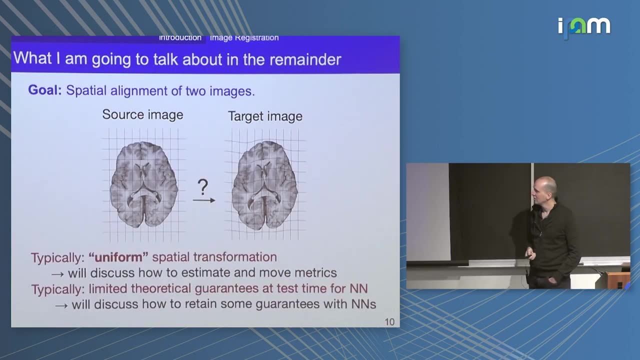 over these regularity of transformations, also at test time and not only at training, And if you construct it in the appropriate way, I think you can do this. So what will I talk about in this remainder of this talk? It's really two things mostly. 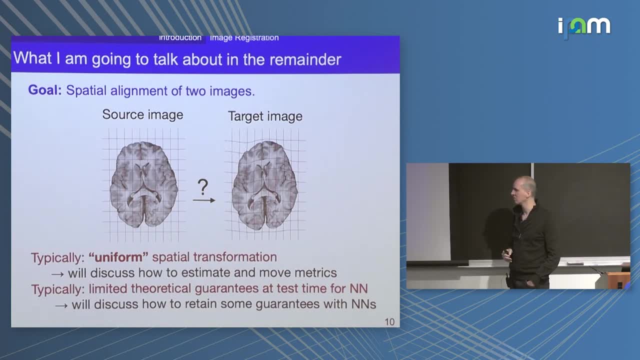 and then a little bit of an outlook and an overview of some other things we've done. First of all, when you do these registration problems, when you try to set them up, in the vast majority of the cases what you assume is that the spatial transformation 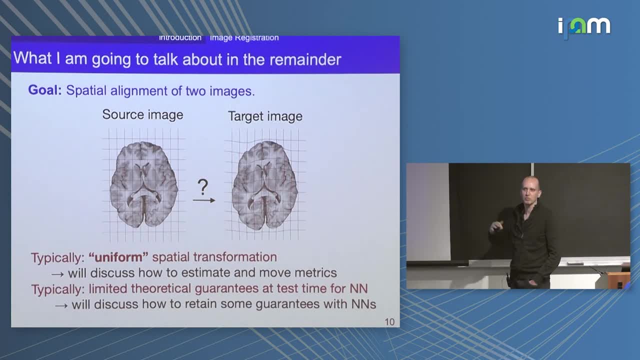 that you're looking for is in some sense, smooth, and it's, in some sense, uniformly smooth, meaning that the smoothness panel that you put on at every location is the same right, And this is a nice model in the sense that it's simple. 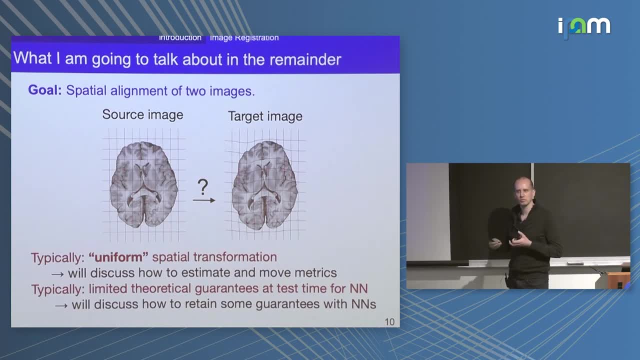 but might not be the most realistic model if you have those like different tissues, or if some parts of the space have a higher desire to move farther than others, And so it might be useful to have models that break this assumption. And then, as I said, typically they have relatively limited. 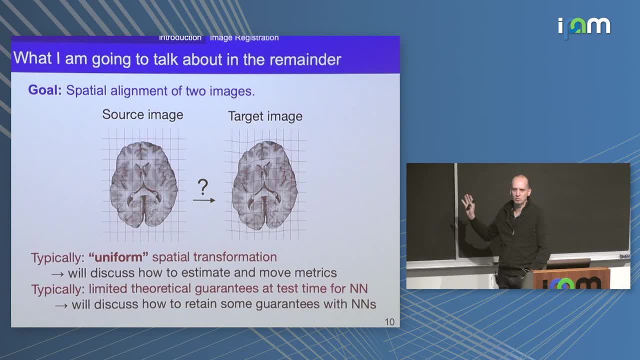 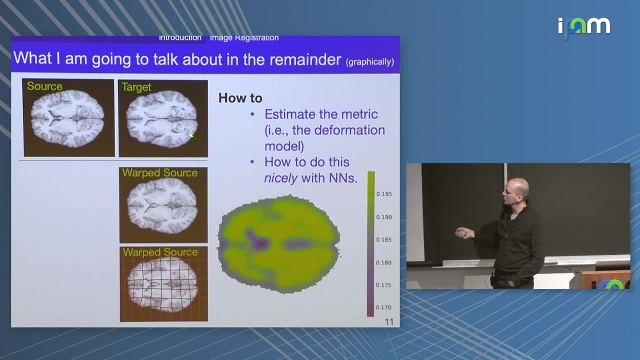 guarantees at test time and I'll try to walk you through one, one possible approach to, of course, others to try to get around this a little bit. So, essentially, what I'm gonna push for is something where you have a source and a target image. 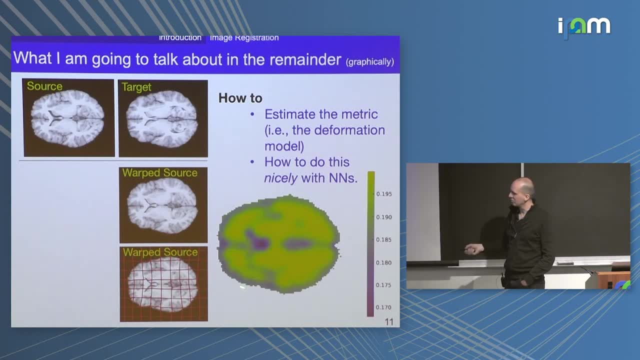 you'll have a warped source and you also get some sort of map of, like the estimated regularity, right, And so it estimates, like the, how space should be locally regularized, how smooth it is, and this comes all from the data that you look at, right. 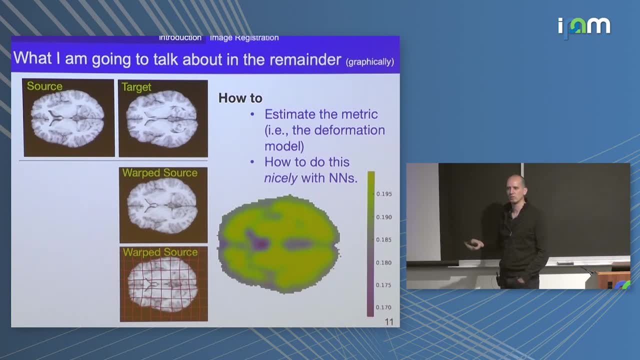 You can probably at this point already appreciate that this is no way something you could do if you only look at it from this paradigm of having one source and one target image. you really need the population for this, because otherwise you have no way to get at this information. 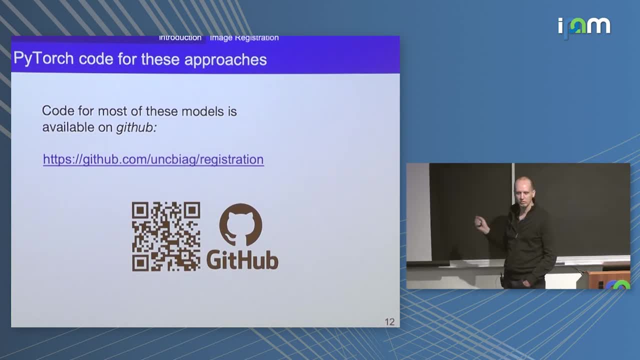 So most of the things I'm talking about here is available as PyTorch code, if you want to check some of this out. Also, there's sort of like a base registration library that implements all of these optimization-based approaches. So let's first talk about parameterization. 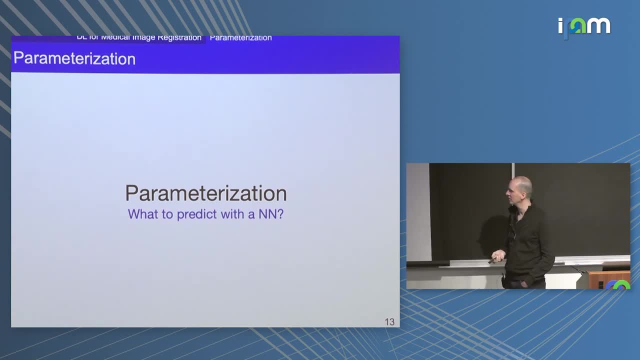 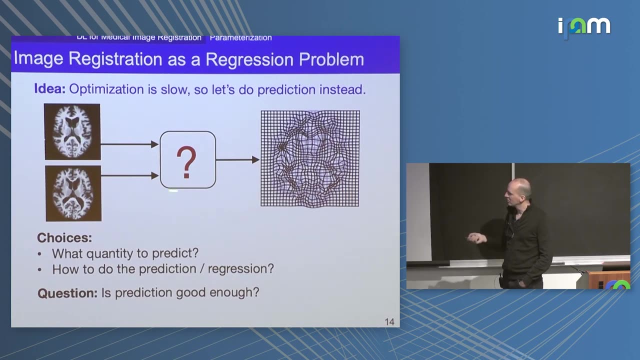 So if you want to predict registration with a neural network, what do you wanna predict? So the idea here is really quite simple. So you have a source and a target image, you go through some sort of black box and out comes your transformation. 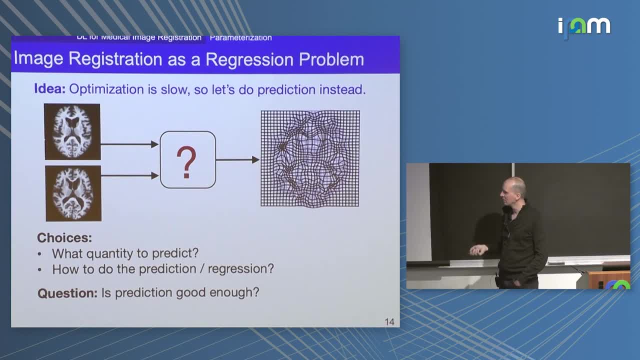 The choices that you have here is, first of all, what quantity you wanna predict, and then how do you wanna do the prediction or the regression, And then, of course, in the end, if the prediction you get isn't good enough, right, Because you can predict something. 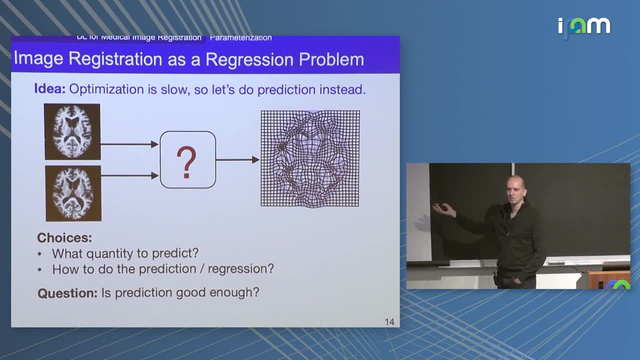 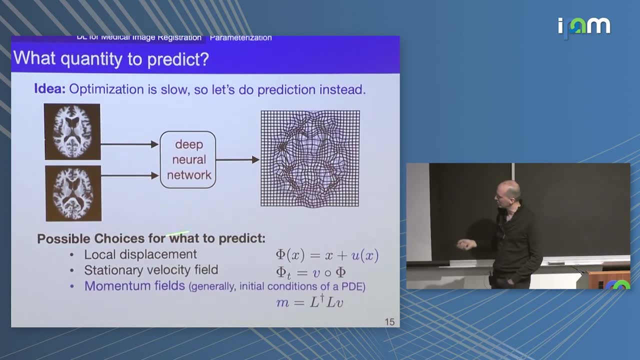 but if it's sort of way worse than what you would get with your classical methods, probably you haven't really won a whole lot, maybe speed, but that would be about it. So what we're gonna do the prediction with, of course, 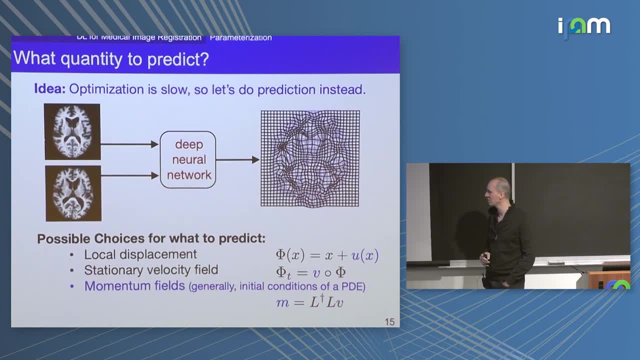 is a deep neural network, but you could probably replace this with some sort of other regression model And the choices that we're gonna consider here. first are these non-parametric approaches to parameterize a transformation, meaning that it's all based on some vector field. 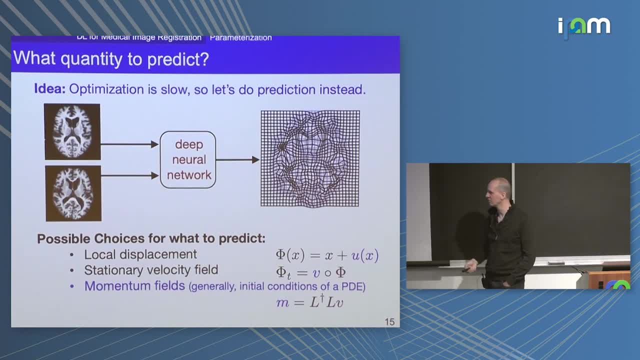 and these vector fields then have different meanings depending on how you parameterize. For example, the vector field could be directly the displacement field that you're interested in. It could be a velocity field that you integrate through, and this integration through the velocity field. 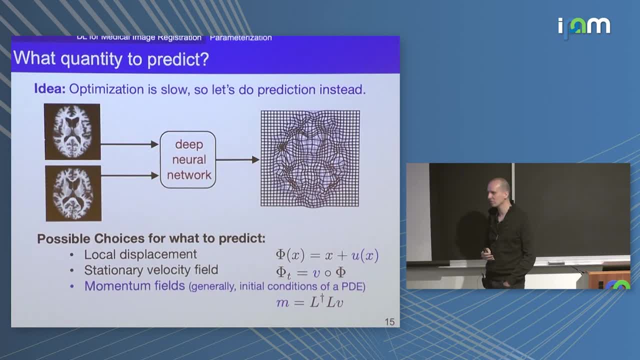 then of course allows you to get some regularities of the transformation, So, for example, to avoid folding if it's smooth enough. or you can go even more indirectly to predict the vector field, something called the momentum field, where essentially there's a vector field. 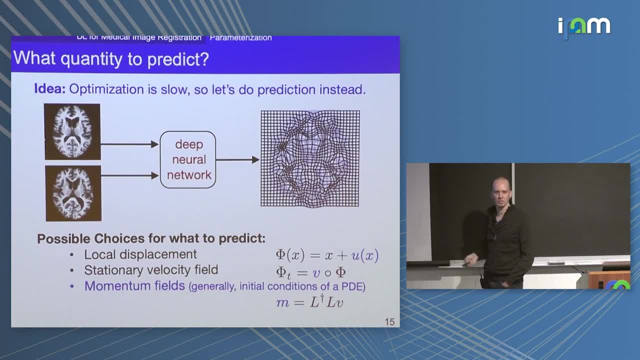 that then gets smoothed to get the velocity field and then you integrate through the velocity field And this is sort of mostly what I'm gonna be talking about. If you've never seen this before, bear with me for a few minutes. I'll give you like a very short intro to how this works. 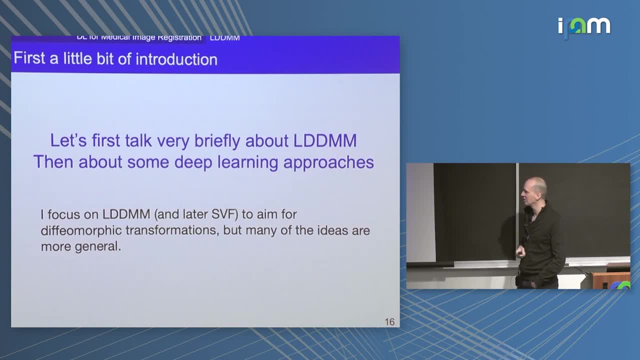 So for this, let's briefly talk about a model called LDDMM, and then, as I introduce this, I'll take a step back later to something slightly more simple, but it's just to illustrate where this is going in terms of how the registration model is formulated. 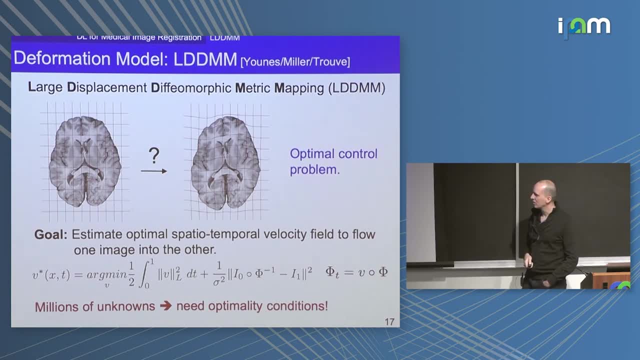 and what kind of properties this may have. So if you look at LDDMM, this stands for large displacement. if you're a morphic metric mapping model, It's actually it's probably, let's see, about 20, 30 years old this model. 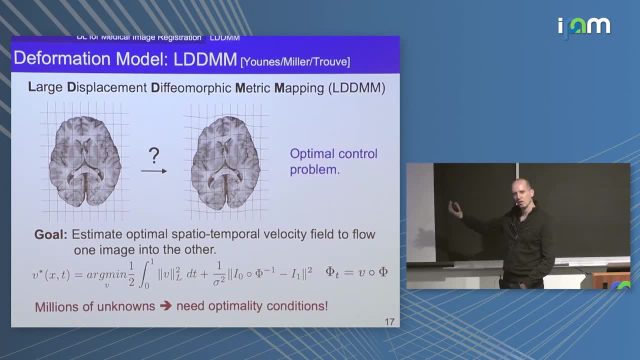 So it's not. it's a nice model because it looks at it from sort of an optimal control point of view. So what's the setup here? The setup is really: you want to find a time-dependent velocity field, so a velocity field that changes in space and time. 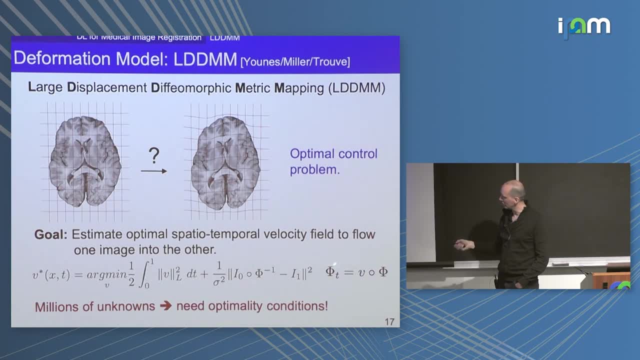 That if you flow along this velocity field, basically just along, according to this equation which gives you the spatial transformation, if you flow along this velocity field at unit time, you can deform the source image so that it matches the target image as well as possible. 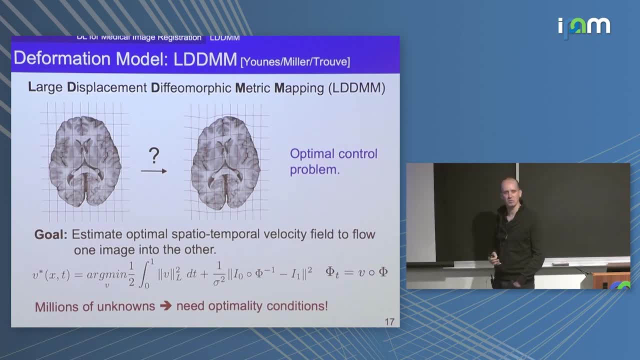 And of course, there could be an infinite number of different options of how you flow. so you need to somehow penalize what you consider a good velocity field, and this penalty is typically some form of like Sobolev norm, and you integrate this over time, right? 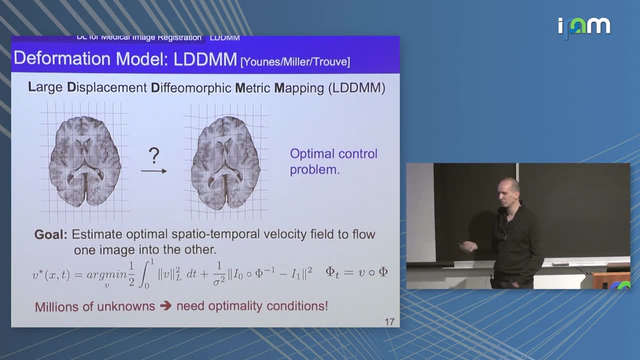 So you want to have in some sense a shortest path. If you see this from the point of view of like driving your car from point A to point B, maybe you want minimum energy consumption so you go at the same speed and don't constantly accelerate and brake. 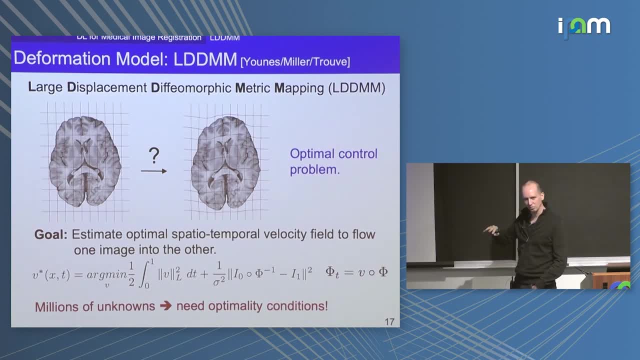 and here it's the same kind of thing. So you have a velocity field and in some sense should be smaller with respect to this norm, and then when you apply this transformation, it should warp the source image to the target image and there's a compromise again between these two terms. 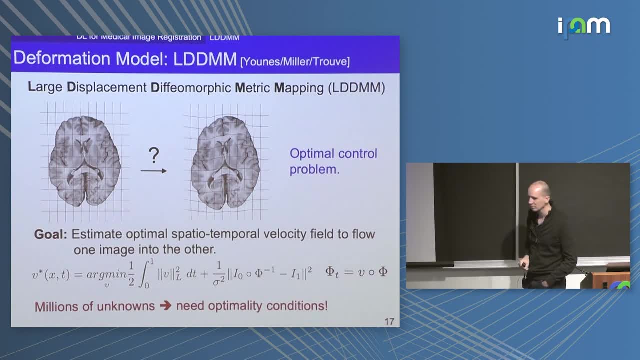 this is the regularity term and this is the image similarity term. If there's anything unclear, please stop me. yes, Oh, can I just for notation. so do you really concatenate v and phi? I mean, like v is the velocity? 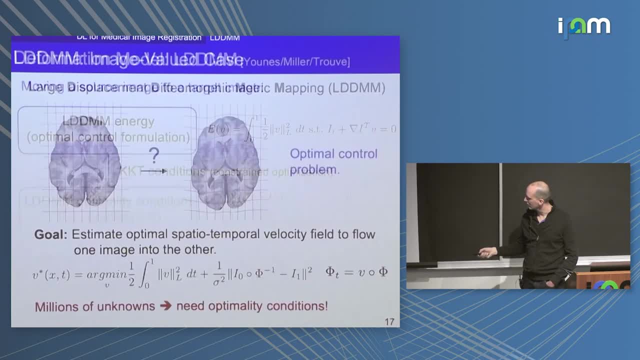 phi is the transformation, right? Oh no, this is just oops, sorry, this is just v sort of v of phi. Oh sorry, this is the notation. yeah, I'm not concatenating them as maps. yeah, 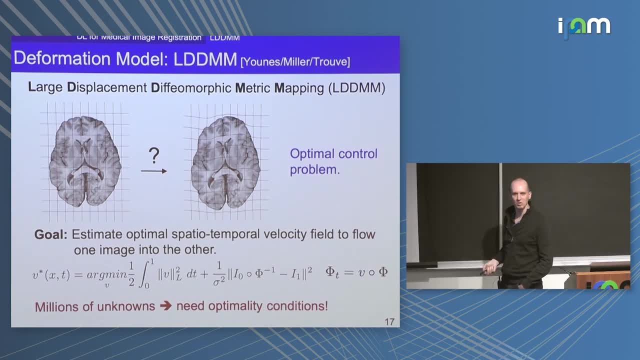 Sorry, yeah, maybe this notation. yeah, Yeah, I'm solving an ODE. Essentially this just means maybe the notation is a little bit unlucky, but essentially it just means you have a point and you flow it along the velocity field. 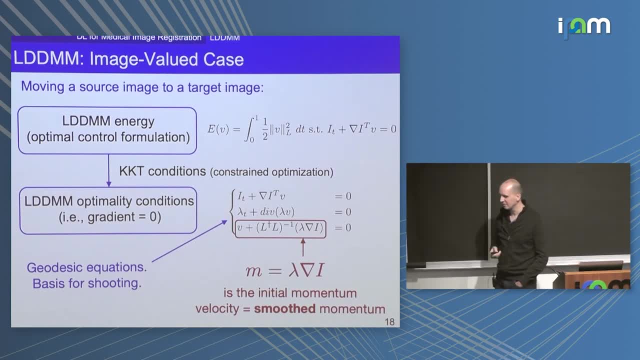 So if you formulate this, I mean you can also formulate this, and I think it's easier if you go about it in this way, where you just say, instead of like solving directly for the transformation, you just say you can just take the image. 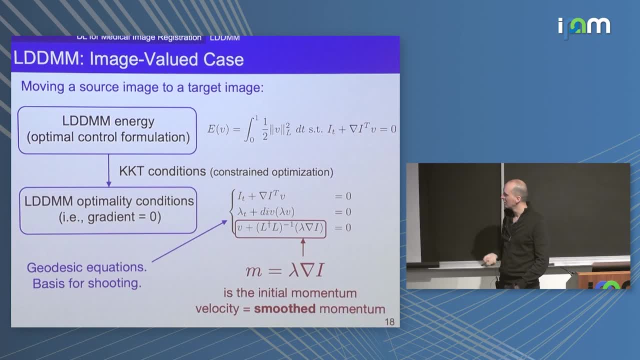 and you flow it according to this advection equation. It's essentially the same, And so, if you start from this formulation, you can compute what the optimality conditions are right. So what do you do? You just compute the first variation. 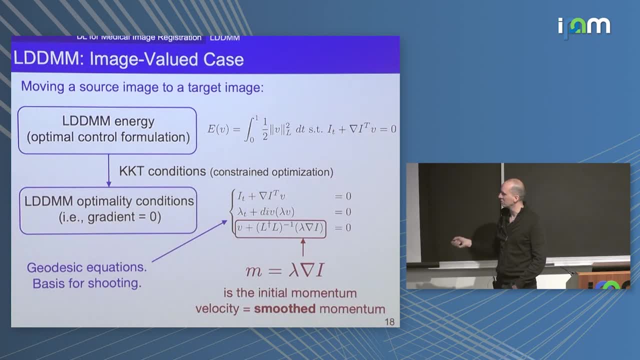 see when this goes away and you end up with this triplet of equations. So the triplet of equations is you have in your forward model, you just flow the image according to the velocity field- Then the adjoint equations. it's just the scalar conservation law. 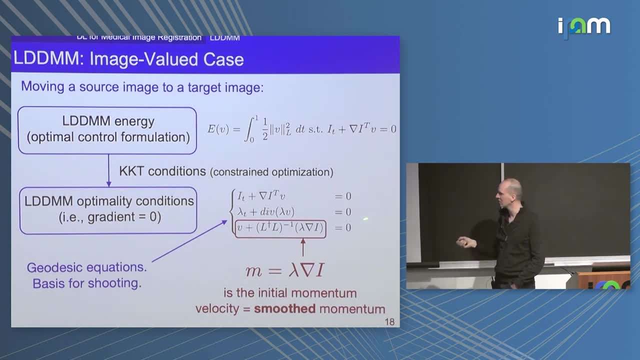 And, if you want to, to look at this from the deep learning paradigm, this is essentially a continuous version of error backpropagation, right? So this lambda is essentially the error that's backpropagated over time, And then you have something that couples. 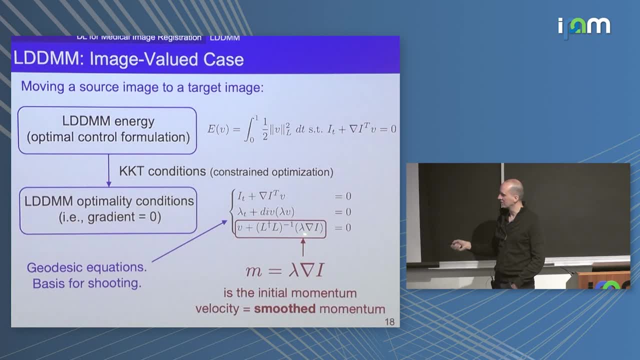 all of these quantities together: the velocity field, the- in this particular case the scalar momentum, that's what it's also called the Lagrangian multiplier, and then the gradient of the image. So there are a couple of important things to note here. 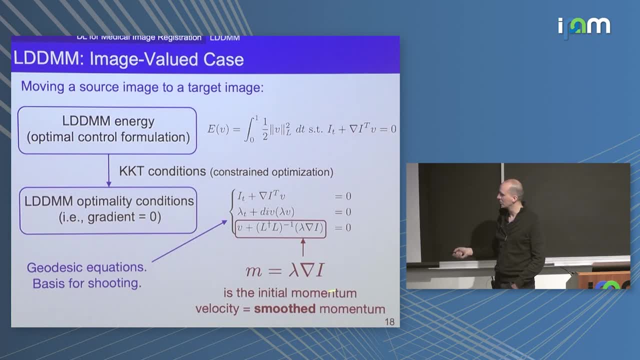 First of all, this quantity, lambda gradient i is also something called the vector value of momentum, And you go from this momentum to the velocity by applying this particular operator And this operator. essentially you can think of it as a smoothing of the momentum field. 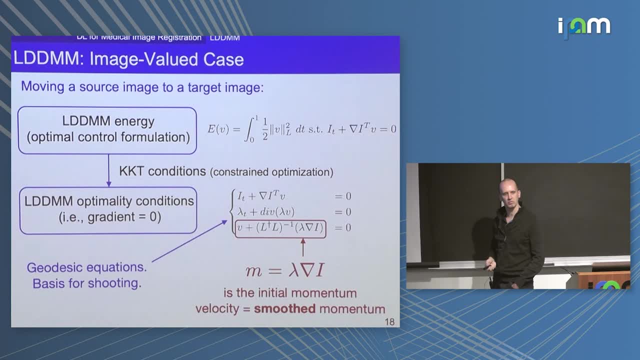 So the velocity field will be very smooth. The momentum field doesn't have to be- And what's interesting about this? also, it can be written as sort of a product between a scalar field and a vector field. So that means if the gradient of the image is zero. 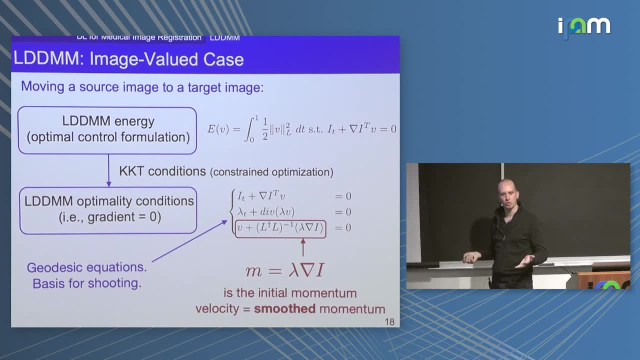 for example, if you would do this in binary shapes, there will be no momentum by construction And at optimality these equations need to hold Subject to some sort of boundary conditions that I have suppressed here, But you can also. what you can also do is you can run. 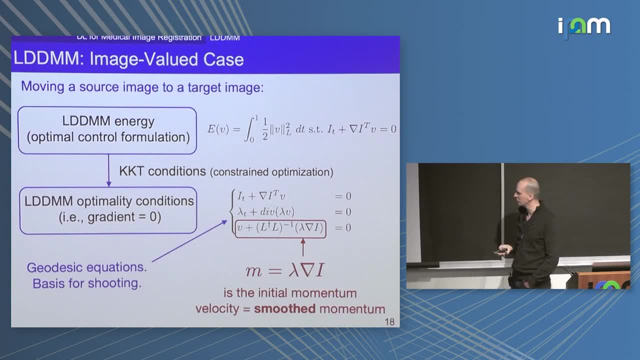 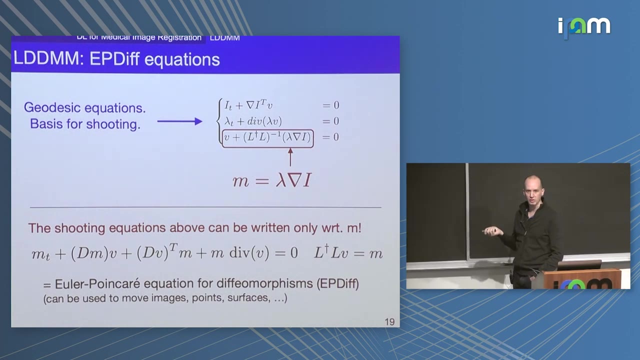 this entire model forward in time, Then it's a geodesic equation for this transformation And essentially, if you know the initial image i zero and the initial momentum lambda, it gives you the whole transformation across time So you can use them for something called shooting right. 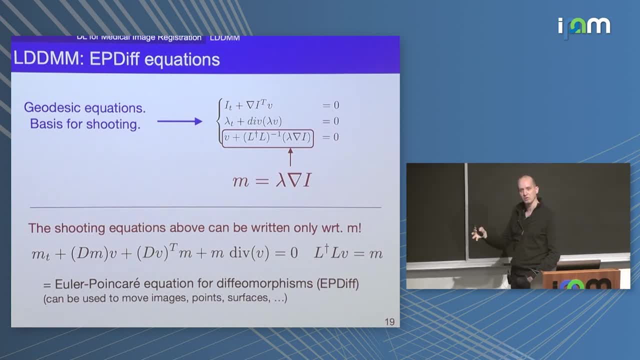 So then, you're not optimizing over the entire spatial temporal velocity field anymore, You're just optimizing over the initial conditions. And what you can also do, which I think is quite interesting- is, if you have this momentum, you can take this equation system. 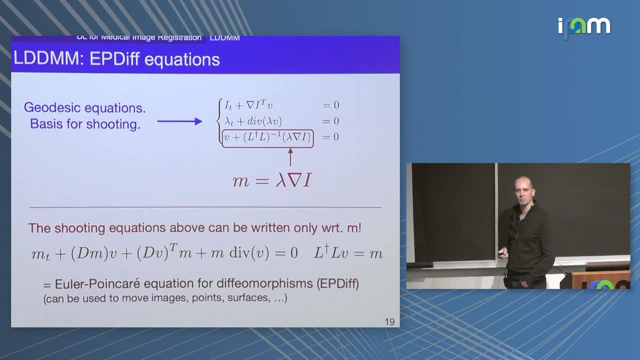 and write it in this particular form, And this equation is something called the Euler Poincaré equation for diffeomorphisms. And then it's only about the transformation itself, Parameterized by this momentum vector field. there's no mention of the image anymore, right? 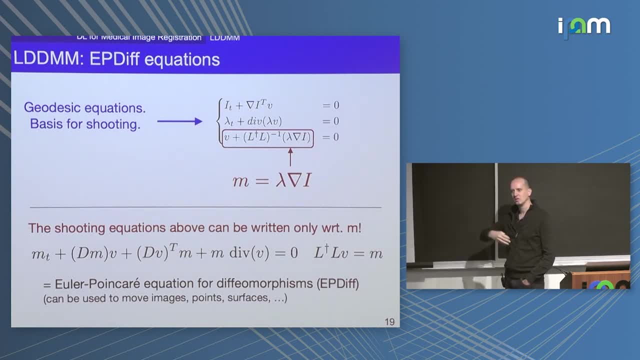 You can use this equation really to describe deformation of space. You can, with the space deformation, move points around surfaces, images, whatever you want. It can be written in this particular form. Yes, So the part L that's coming from the 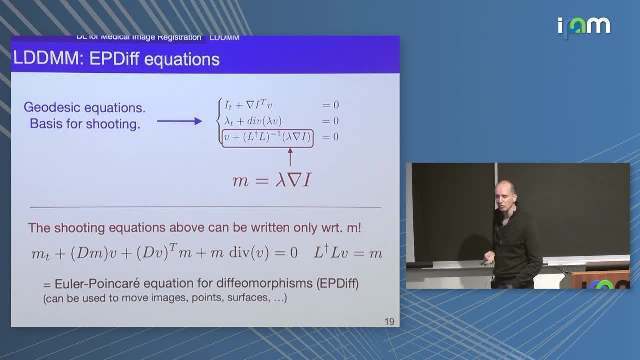 Yes, yes, And in that case we end up with the integral equation in this case. Sorry, what Integral equation in this case? Into what equation? The L? Oh, this dagger, Yeah, Oh, it's just the adjoint. 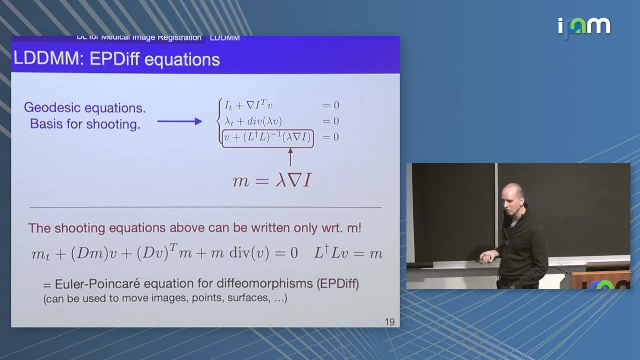 So that means the actual calculation is based on the integral equation or No? so this is a differential operator, right? So it could be something like first derivative minus two times the second derivative. But in practice what people oftentimes do is because V is given. 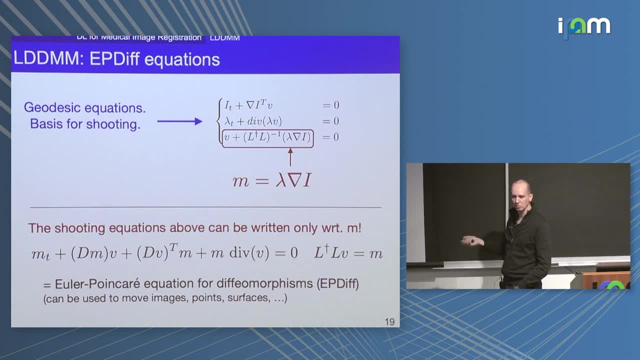 as the inverse of this operator applied to M, and it's a smoothing operator. oftentimes the starting point is that you just assume you have a momentum field and then you smooth it with a Gaussian or a multi-Gaussian, for example. This is what I'm gonna do later on. 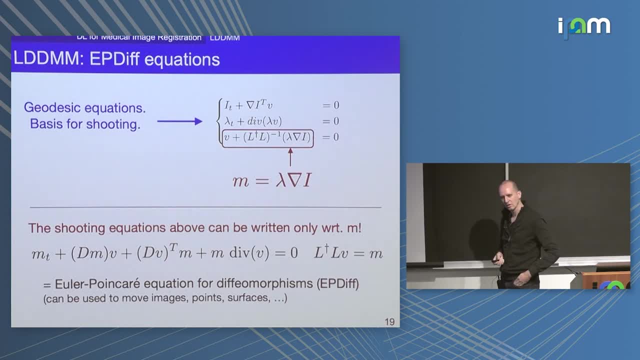 There's no integral in this, It's just the-. Okay, so there is a differential, but with the other data together it'll be like some kind of filter. then, Yeah, it's a filter, exactly, And essentially the filter is, if you take the inverse, 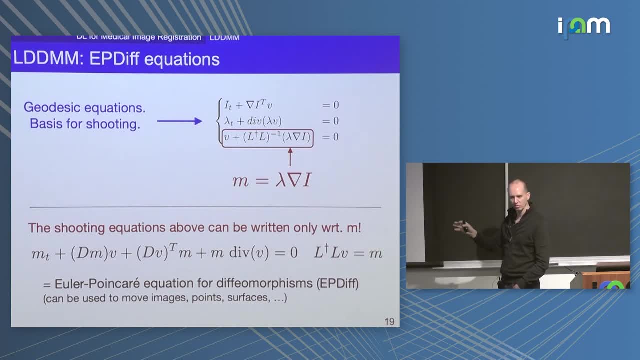 and if you apply this inverse of this operator to M, it will be a smoothing operation, And so oftentimes you just start by defining the smoothing operations in this particular setup And, as you'll see later, I'll essentially use a multi-Gaussian. 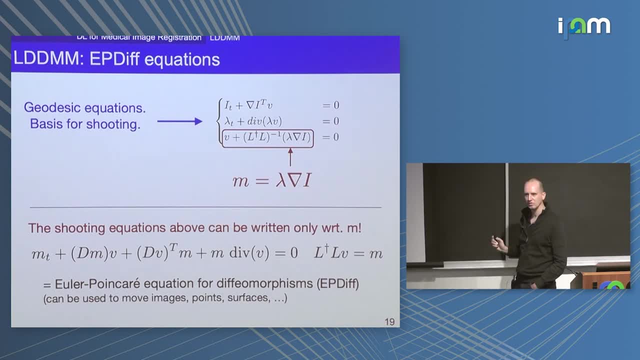 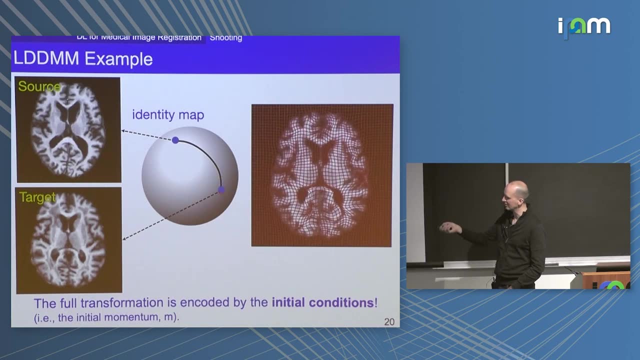 so a mixture of Gaussians for smoothing? Okay. Other questions: Okay. So this is what this looks like, for example: right, You started the identity map, but then you move in some sort of- I mean, this is not a sphere of course. 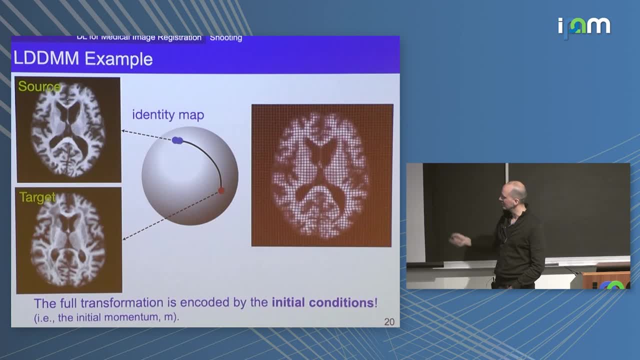 You move in some sort of space and so you can express this deformation of space just based on initial conditions, right? You just imagine like in a simpler case: if you have a line, you just specify the initial slope and you know where the line goes. 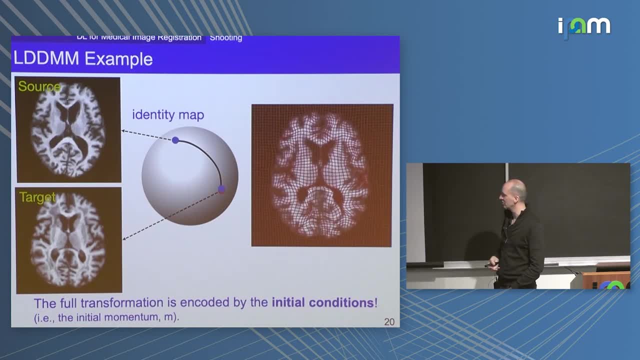 Here you specify the initial momentum and it parameterizes the transformation. And the nice thing is if you're smoothing it sufficiently enough. so if your differential operator is strong enough, then at least in theory you should get diffeomorphic transformations. 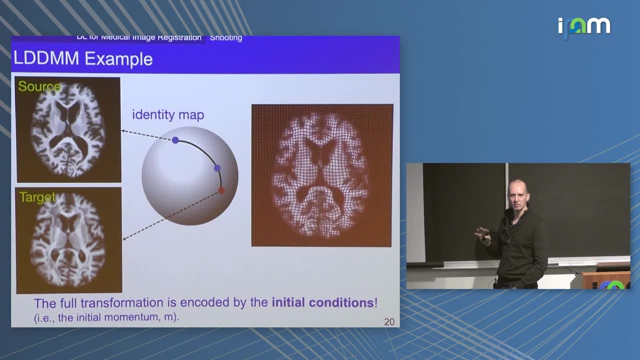 no matter how far you integrate it out In practice. I'm saying in theory right, Because in practice at some point there comes the point where you discretize this and the discretization may wreak havoc there a little bit. but let's just assume we have the perfect discretization. 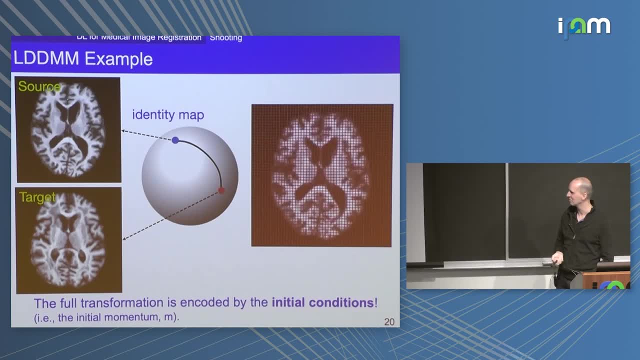 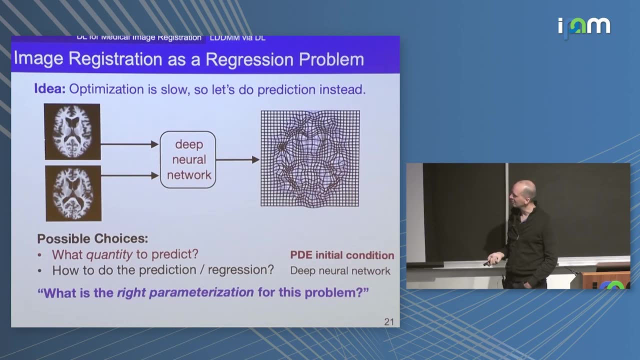 and the theory holds and everything stays diffeomorphic. So everything is encoded in the initial conditions. So now you want to. I guess the prediction that the what we're gonna try to do here is we predict the initial momentum of this LDDMM, the vector momentum. 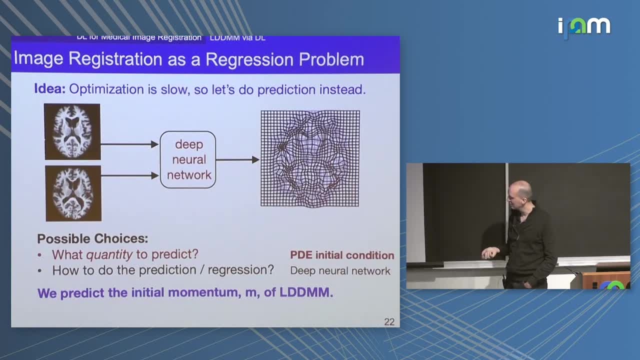 and the nice thing, the nice property this has, if you do this, is that you predict it, but then the velocity that you get is obtained from this momentum by smoothing, and so you do this after the fact, right, No matter what the M here is. 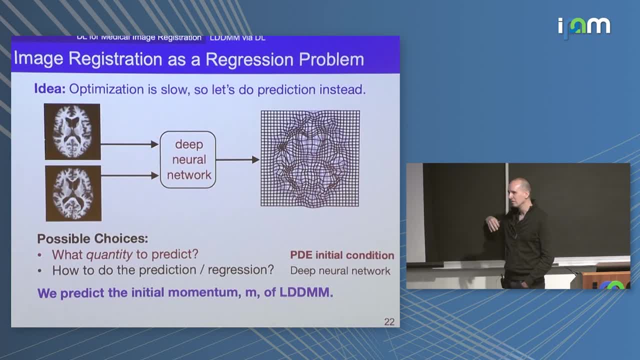 if you predict it reasonably well, the neural network doesn't need to learn about the smoothing. The smoothing comes after the fact, and then you integrate the equation out. so you still sort of retain these properties of getting diffeomorphic transformations at test time. 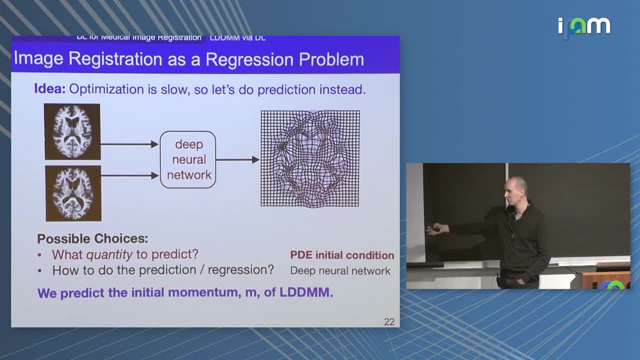 not only during training, because you're not going directly for the prediction of a displacement field, for example. You're going for the prediction of the momentum, and things happen after the fact. I'll give you a little bit more intuition of what this means in a second. 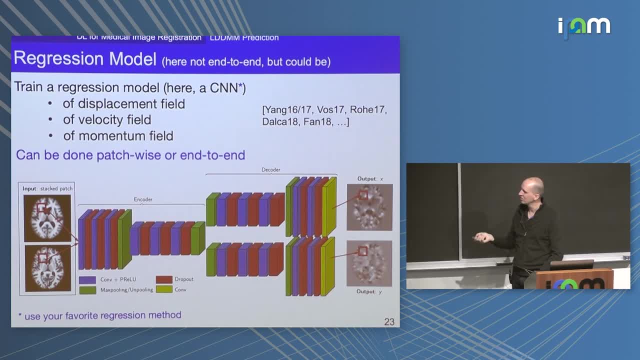 So if you would want to see if this matters, I mean, you could just stick it into your favorite neural network. I mean, this is sort of like the first one we tried back in the days, but you could use something different. and then we have source image, target image. 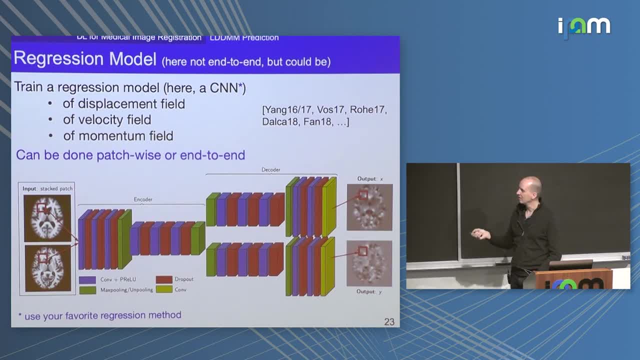 You can do this with patches, or we now do it with the entire images and then you predict these vector fields: right Vector field, either displacement field, velocity field or momentum field. In our case, we'll predict the momentum field. 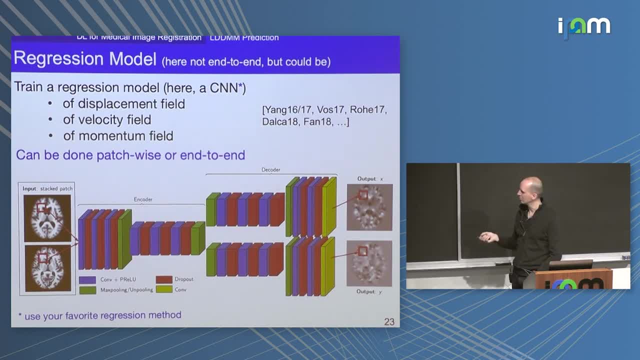 and then what's sort of like hidden here is you would integrate the PDE out, and if you train it end-to-end, then the PDE itself becomes part of your overall model and you back-prop through the entire thing, right? Something like this, I mean. 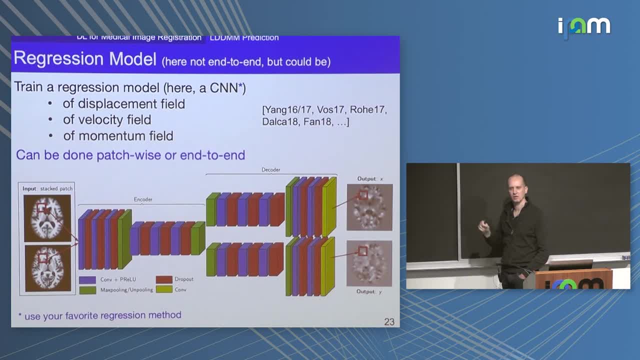 to come back to my point earlier, something like this. I would not want to manually write down the optimality conditions for, but if you do it with PyTorch or probably with TensorFlow, it's not a big deal, You can do it. 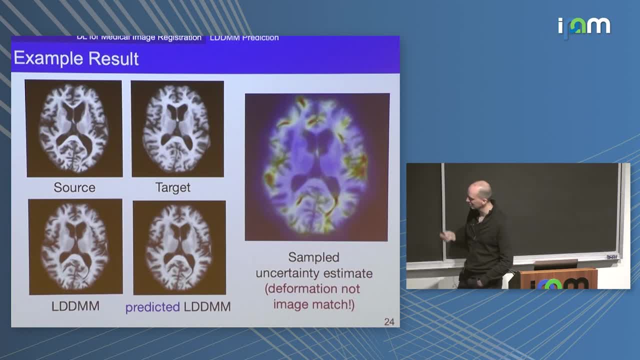 So does this work in practice? Well, here's an example 2D result, and I'll have this 3D result in the next slide. This source image, target image. this is one LDDMM result, maybe not the perfect parameters. 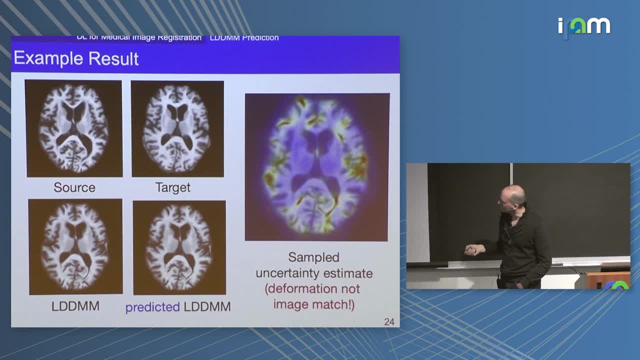 but it sort of pushes the source image reasonably close to the sorry, reasonably close to the target image. and then, if you predict it with LDDMM, with the model that I just talked about, in this particular case, with patches, you get something that looks very close. 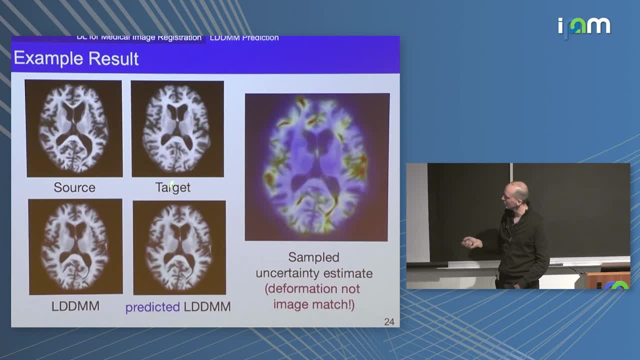 but because this is sort of a funky image here in comparison it's not perfect. if you want to, you can do some sort of sampling. so we did some sort of sampling of sampling with dropout here. then you get a bunch of predicted momenta. 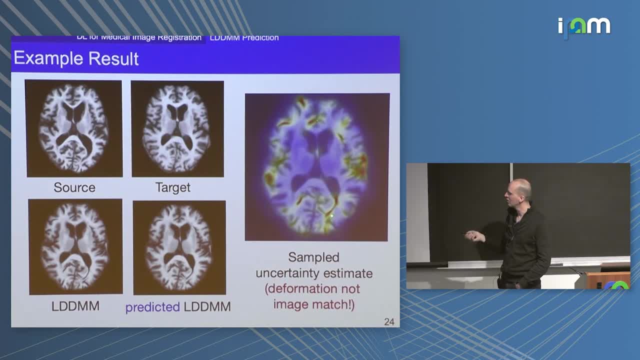 Integrate this bunch of predicted momenta out and then compute uncertainty maps Like blue you're relatively certain, Red you're pretty uncertain, And so it highlights, I think, regions that seem to be reasonable where maybe you should be a little bit cautious in this prediction. 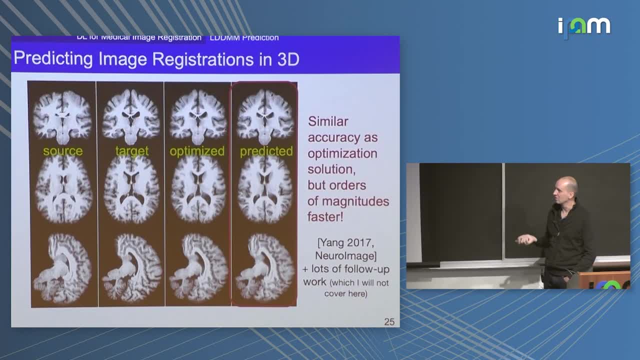 So you can play these kinds of tricks. You can also do this, as I said, in 3D. The results are very, very similar, at least visually- You'll see in a second also quantitatively, to the optimization result, where you really 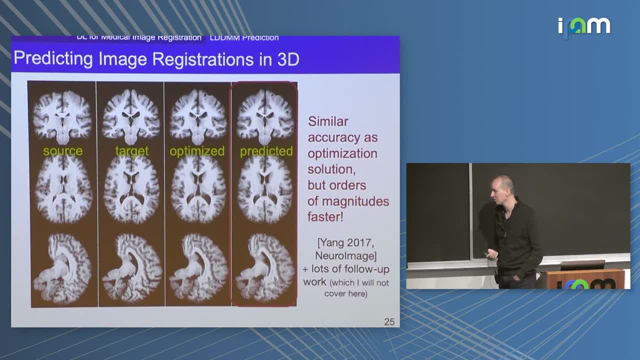 do this very high-dimensional optimization over this initial vector field for the momentum, But it's orders of magnitude faster. So maybe before you required like 10, 15 minutes on a GPU, You can do this now in a few seconds. The thing, of course, is that it's in reality. 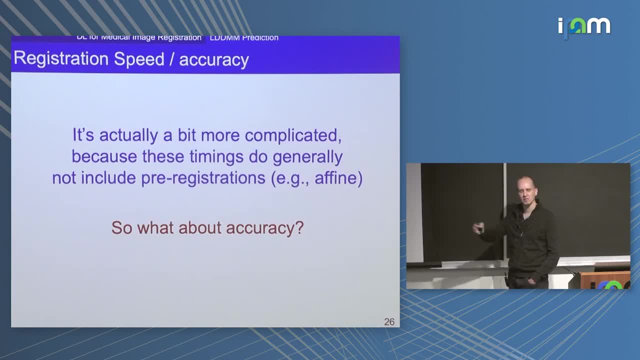 a little bit more complicated, because you talk about these models And this deformable part is now very fast, But maybe your bottleneck is now the affine registration. So, that being said, I have to say that I'm not really talking about this. 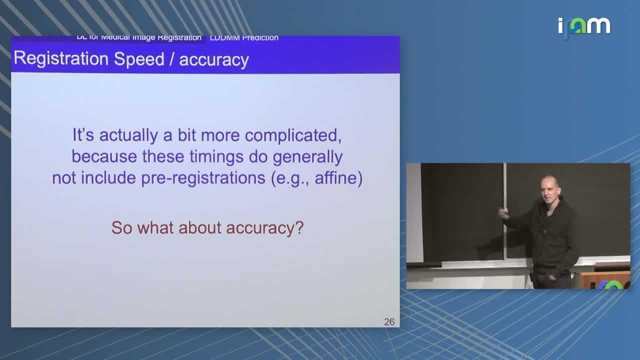 But you can also, of course, have models that predict your affine part, And then you can do everything fast still. You can integrate this, But the thing is that these deformable registration models are faster than typical affine registration when you do optimization. 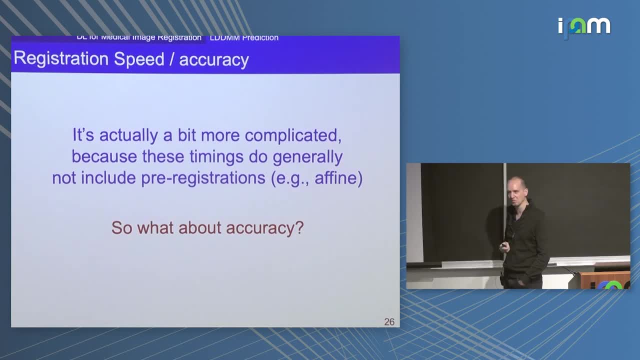 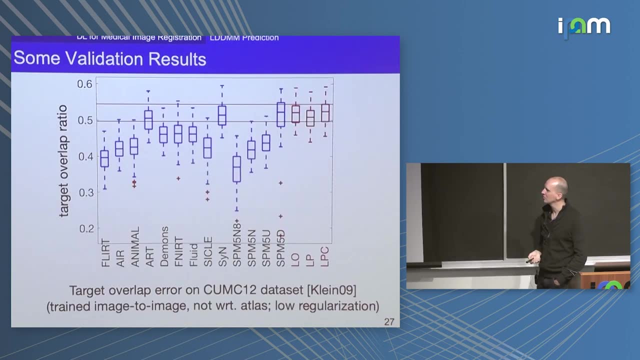 So you may need to worry about other problems in your processing pipeline. So what about accuracy? So we did some sort of, We did some sort of evaluation on one of these, actually on four different data sets. I'm just showing you one here. 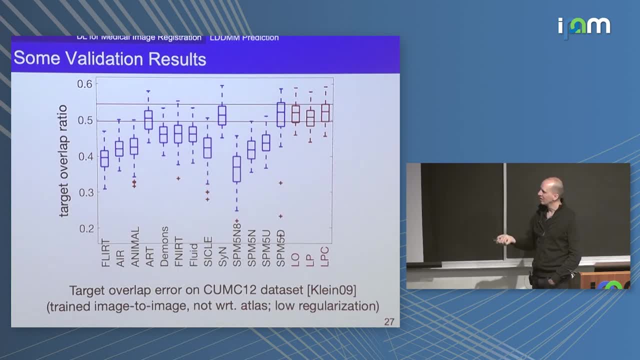 These are different registration algorithms. This is brain registration on the y-axis target overlap ratio, And these red ones are sort of always optimization-based. LDDMM. LP is with this prediction And this is with an additional correction step, And what you see here is that it essentially 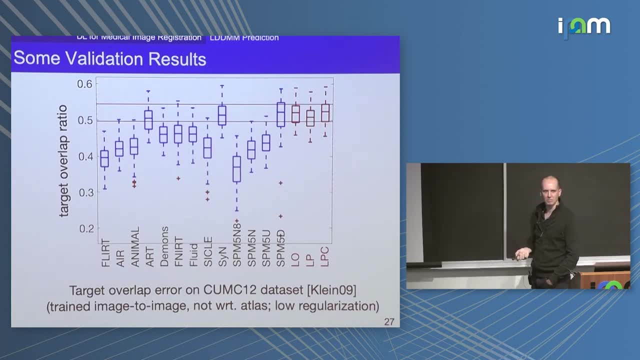 gets results that are similar to state-of-the-art optimization based algorithms like SPM or ANTS- Actually, ANTS is the syn here, But what you also should see is that this performance of these algorithms, at least on this particular data set, 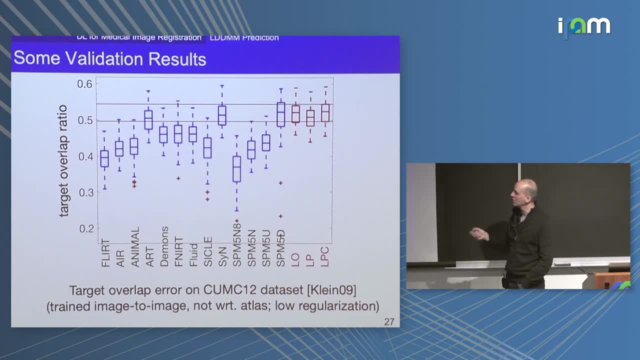 they are all not very good, right, Because ideally it would want to be at one which is somewhere up in the roof here. And these algorithms, they do a decent job at registration, but they're not perfect And I think there are two possible reasons for this. 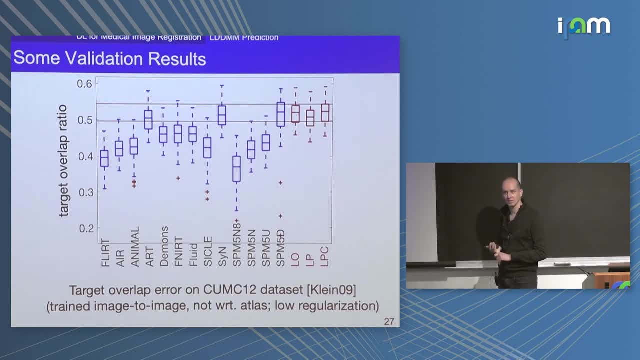 One reason is that the manual segmentations are probably not perfect. They're a little bit, They're a little bit noisy, But probably also these algorithms don't really achieve perfect registration results because some of these registrations are in fact difficult. 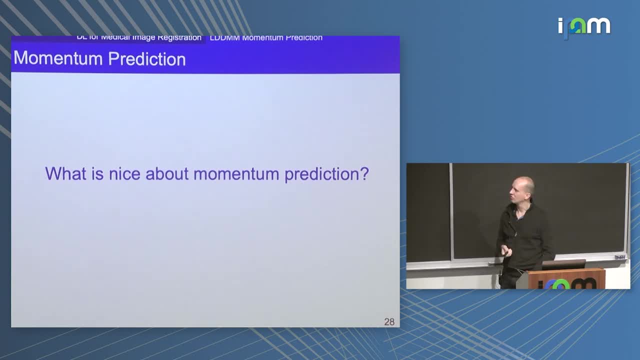 So maybe let's take a little bit of a step back and talk about what is nice about this momentum prediction in the first place, I told you one particular nice thing: that if you do smoothing after the prediction of the momentum, at least in theory, can retain some. 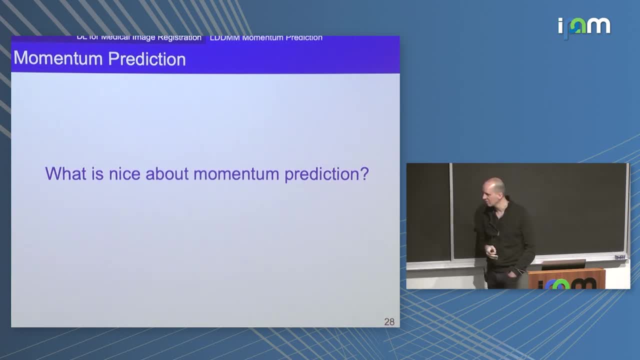 of these theoretical guarantees that you still get diffeomorphic transformations. Performance-wise it looks like it's OK. right, But not something necessarily that blows me out of the water. I mean it's fast, but it has similar kind of performance. 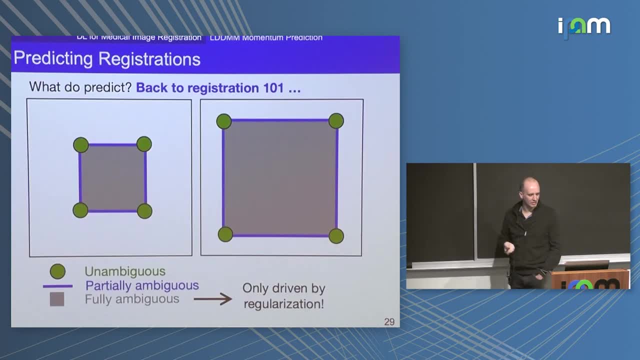 But let's take a step back and see why predicting momentum may be a nice thing to do. So if you look at one-on-one registration, let's say you have this gray square, small, one big one. You want to register them to each other. 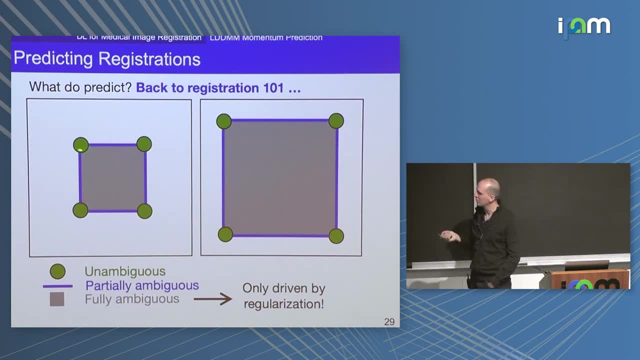 Then the points that really, I would argue you don't have a big issue in terms of finding correspondences, are the corner points. The edge points are already a little bit. It's a little bit ambiguous And whatever happens on the inside is entirely driven by the regularization right. 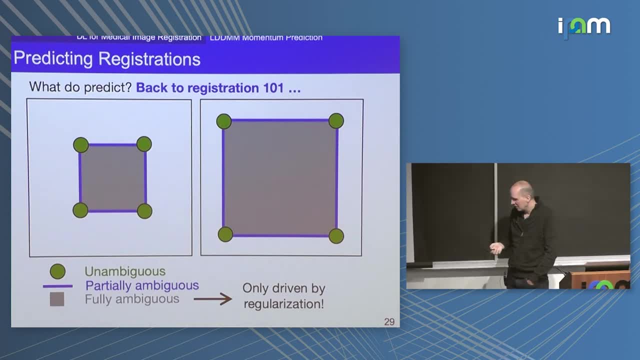 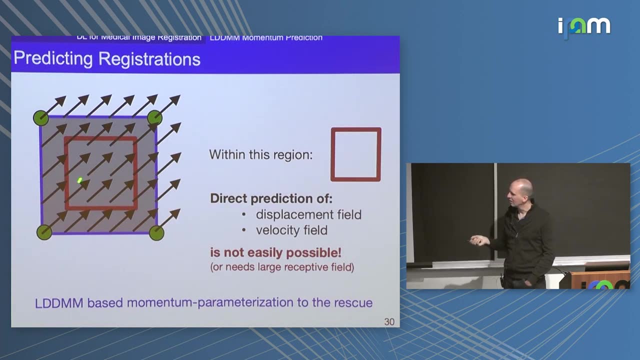 It's the famous aperture problem. And so why is this an issue when you do predictions? Well, if you would have some sort of displacement field that's everywhere and you just predict based on a little patch, because, let's say, you predict patch-wise. 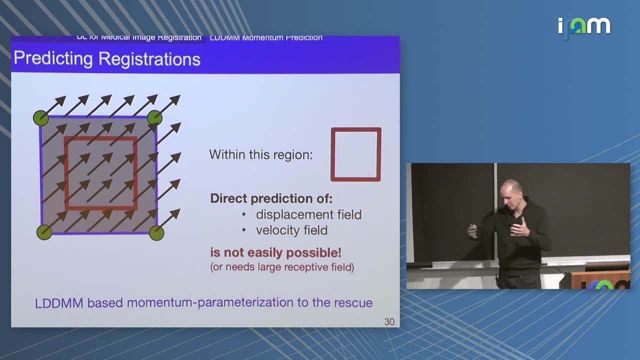 so maybe your region, where the network looks, based on the size of the filters you have and the network is relatively small, then it's difficult. It's difficult to predict something in this particular just by looking at information in this particular region. right, because you don't have enough spatial context. 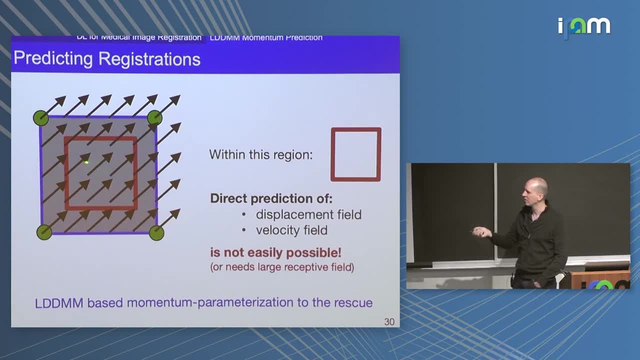 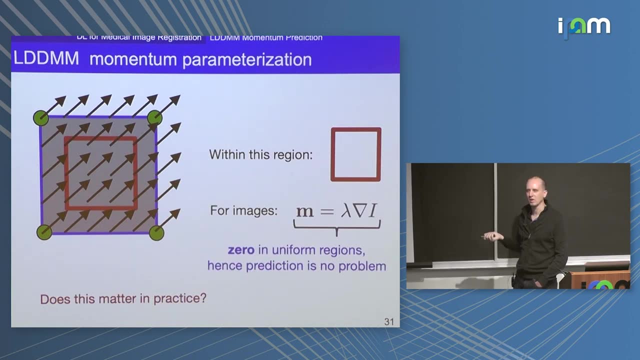 So it's not easily possible if you would directly want to predict displacement of velocity field based on this little patch. However, if you do this with the momentum, there's no real issue, right? Because, as you might recall from what I described earlier, 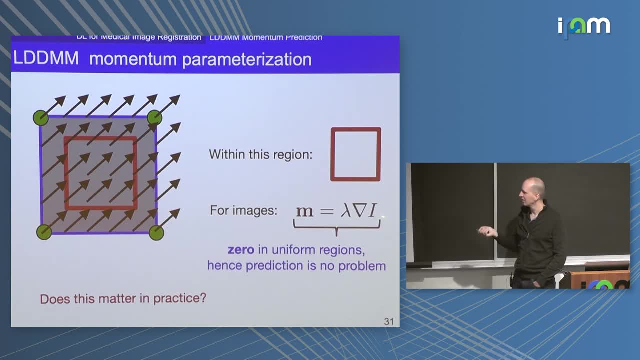 this vector. momentum is a product between a scalar and a vector, So I don't really know what the scalar is, but I know that in a uniform region this gradient is zero, hence the momentum is also zero. So if you're in a uniform region, 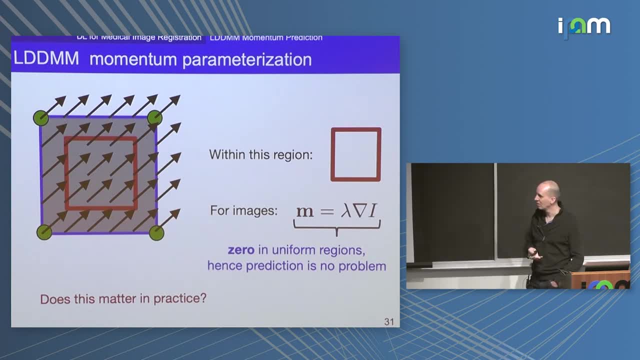 you don't really need to worry about predicting momentum, because you can just predict zero. If you're in a region with texture, then it's fine right, Because in a texture you get some sort of information from the image of what might possibly correspond. 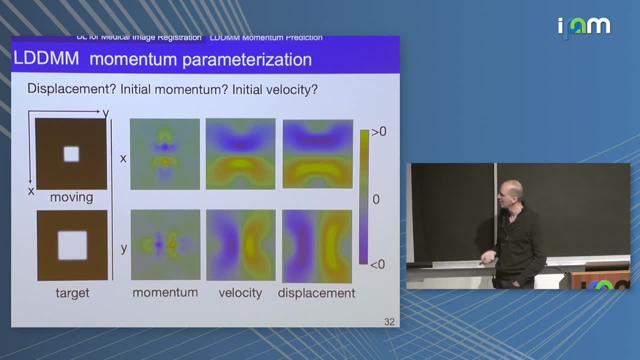 So that's useful. So if you look at this in a practical application where you look at this registration problem from here to here and you look at what the initial momentum is, ideally it should only be supported on these edges. It's a little bit smeared out numerically. 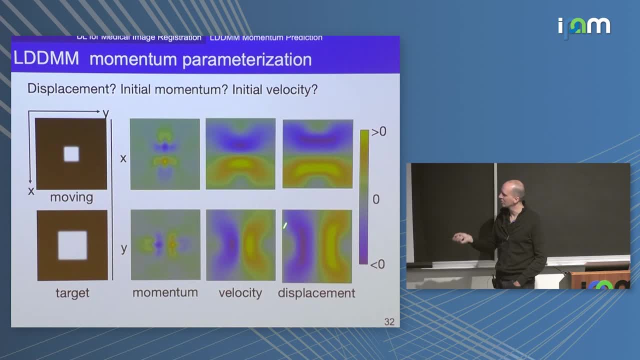 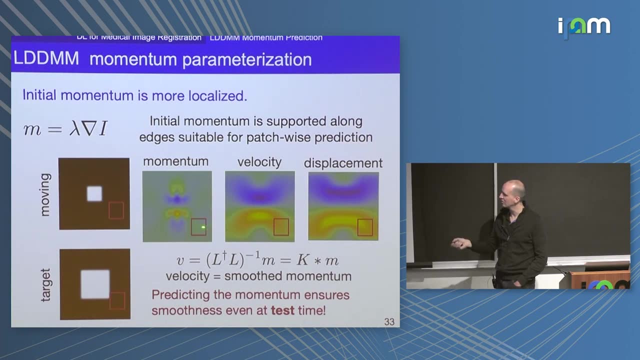 But it's momentum, x and y component, velocity, x and y component, displacement, And then if you would just want to predict it based on this patch, then you see, for the momentum in this area at zero, for the others, because it's smoothed out, there is some sort of value. 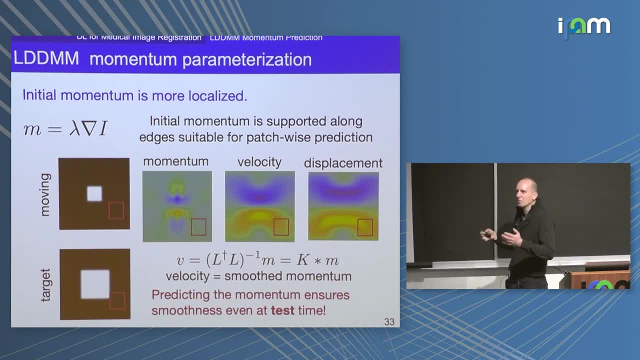 but you can't really predict this easily, right? So to make this maybe a little bit more concrete, I would imagine- and we haven't really done this- I would imagine, if you do this on natural images, like brain images or lung images or whatnot, 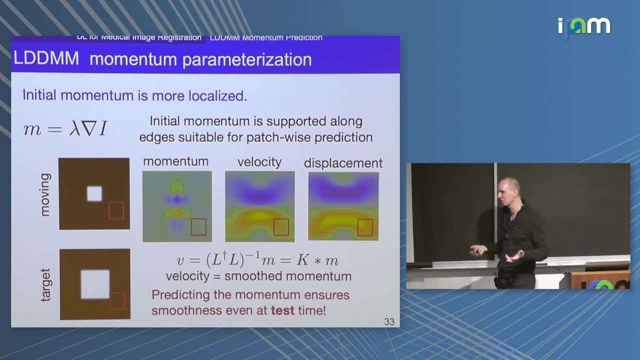 it probably doesn't really matter that much, because there's always some sort of texture going on. But let's say you would want to deal with images that are represented as binary images, so essentially shapes I could imagine, though I haven't done the experiment. 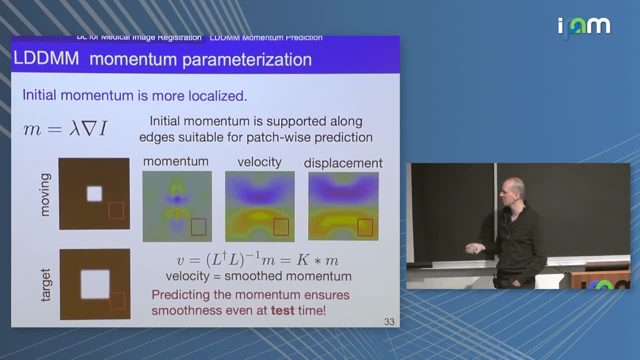 that you run into issues when you would want to predict displacement fields or velocity fields, because you just don't really know what to do. So The nice thing, The nice thing then, is if you predict the momentum here, you can predict zero and then all the regularity. 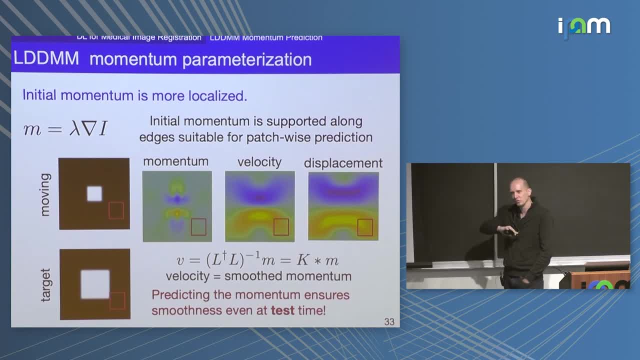 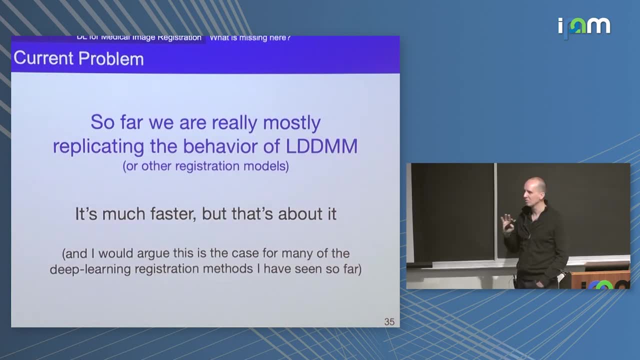 that needs to happen just happens also at test time, because you smooth it after the fact. So it all sounds pretty good, right so far. But the problem is that so far we're really only replicating the behavior of LDDMM or other registration models. 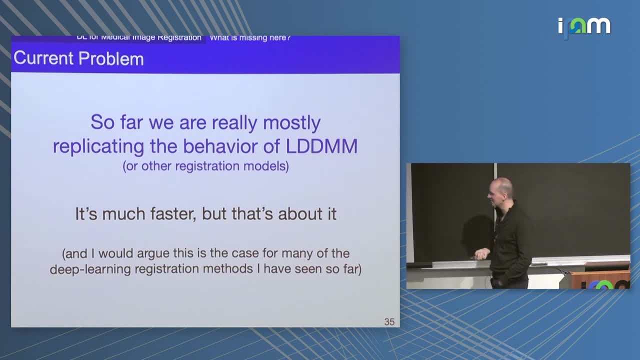 It's faster, great. I'm very happy about the fact that it's faster, but that's about it, right? So the performance is not that much better at this point, And also, so the question is: can you do something a little bit more interesting, right? 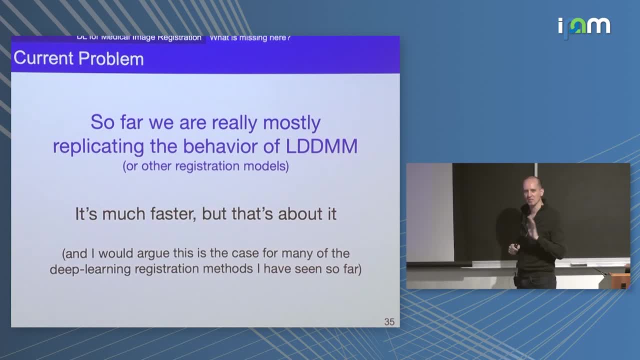 Either increasing the performance- and I think you can do something about this, I have one slide a little bit later that points in this direction- Or maybe create a more flexible model that, even though the overlap measures may not be better, at least tries to tease out some additional information. 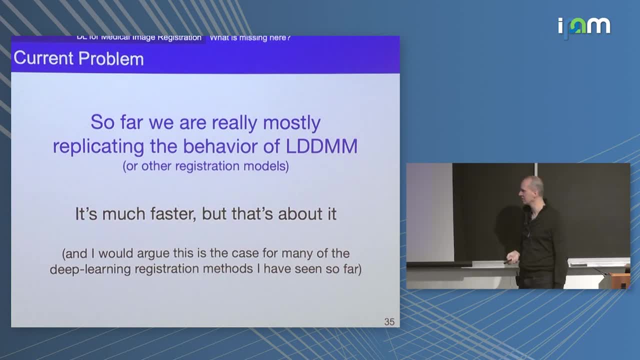 that other registration models may not have available in this sense. So I'm going to drive towards this. So for me, LDDMM is sort of a nice model. but yes, Quick question: So far, what is your loss function you're using? 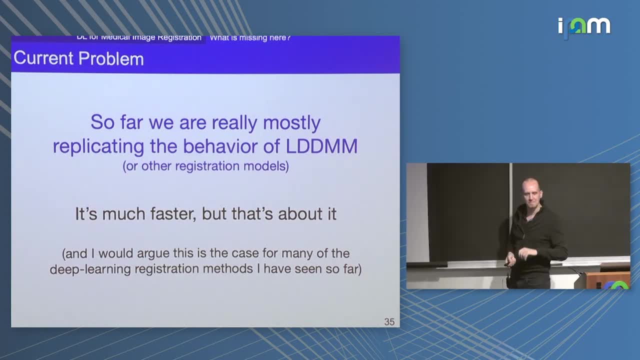 Are you trying to really? Do you replicate LDDMM or you have an image similarity as a loss function? So far, the loss function is really the LDDMM loss function, meaning there's an image similarity term like normalized cost correlation or sum of square differences. 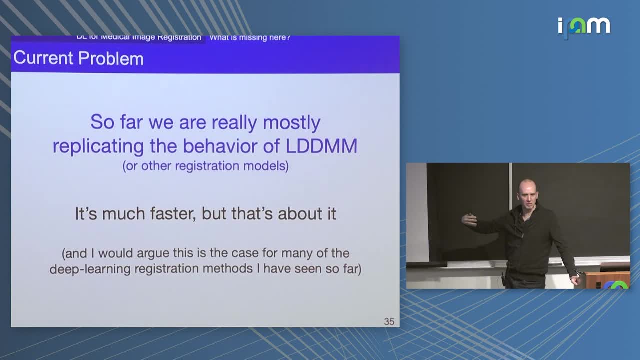 But then there's also some sort of loss on the momentum itself. So essentially this Sobolev norm I didn't just define sort of like an additional condition, just to make sure it doesn't try to predict some sort of crazy initial momentum. 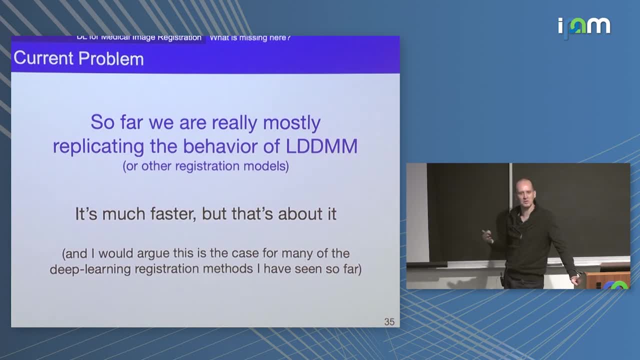 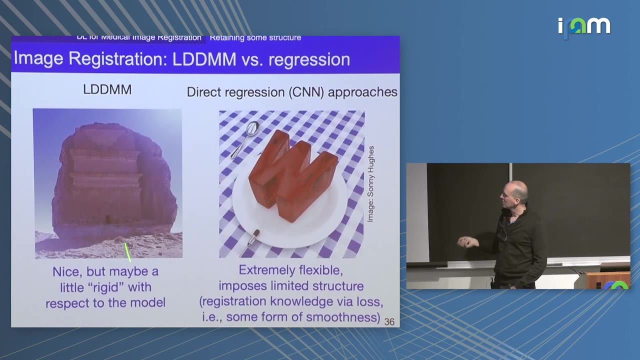 But this is the loss function, Essentially from a deep learning perspective. you could say it's rather boring, right? Because you have the same model that you always had and you just predict the initial condition for it. Other questions. So for me this LDDMM model is a little bit, I mean. 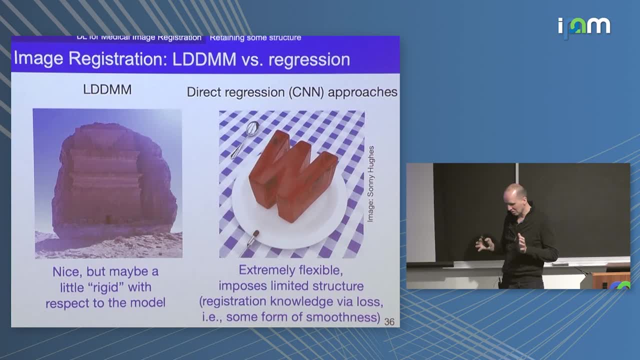 rigid in quotes because it's a fluid model. It's sort of like a nice mathematical model, but you sort of stick to the model. If you were to directly do some sort of regression approach, that's nice but maybe sometimes a little bit too flexible. 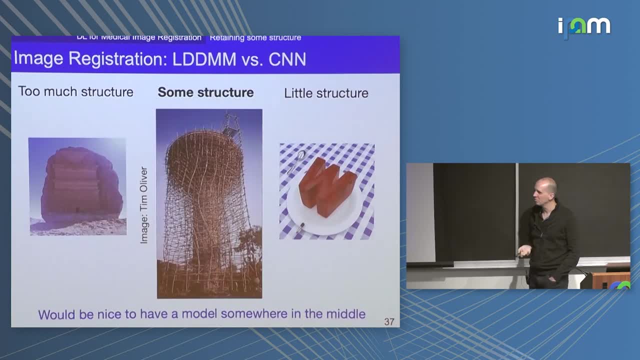 I would imagine, because it can just do whatever it wants. So what I'm going to do is: I'm going to do this. Where I want to be is somewhere in the middle right. I want to build some sort of scaffolding of saying: 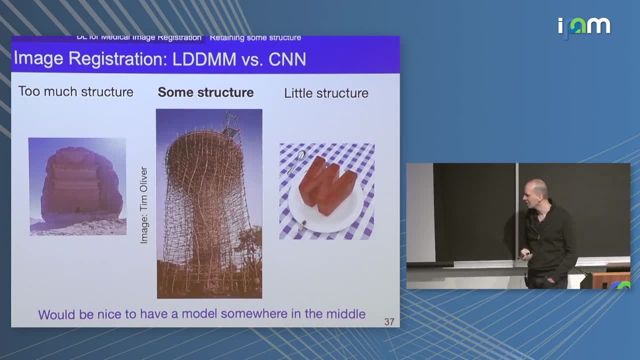 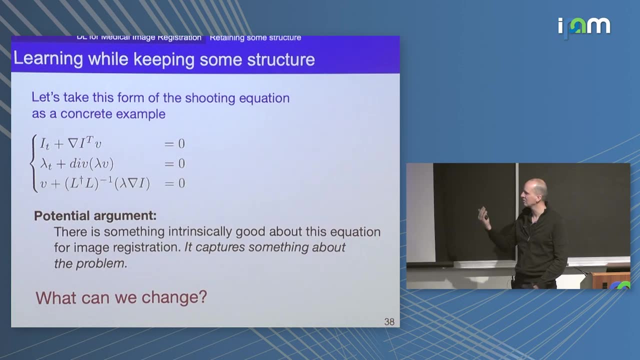 I have a model that I'm reasonably happy with. maybe not totally happy, but I want to change something right, And so if you go back to this model, there are different things you could change right. I mean, you could probably do things. 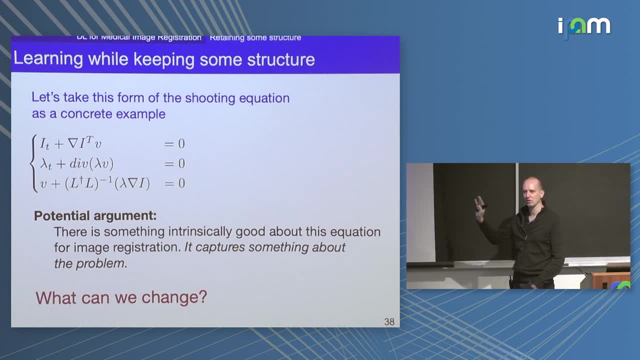 like when you talk 10 of these reconstruction talks. people talked about these variational networks where they essentially unroll some sort of iterative scheme. You could probably do something with this too. That's not what we did, But you could also change out other parts. 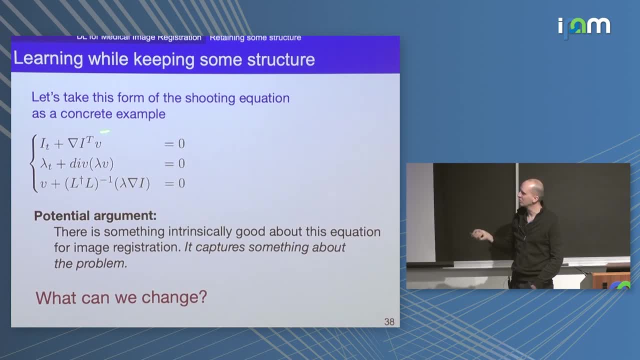 of this equation Right. So I would argue that the first equation is probably relatively uncontroversial, because this is just how the image moves around the velocity field. I don't really see why I would need to learn this. The other equation is sort of directly tied to this. 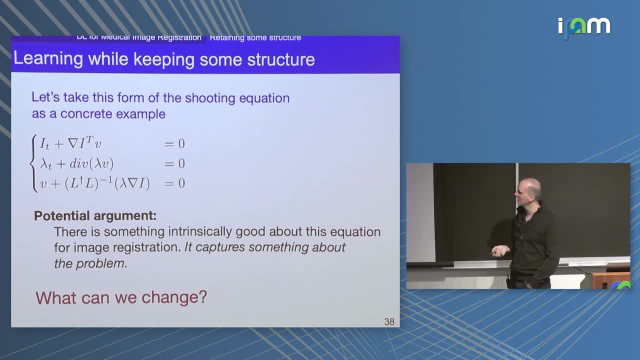 because it's the adjoints, I'm not really sure something should be learned either. So the natural candidate then is this third equation, in the sense if some aspect of it could be learned, And the natural thing to try to start learning is this regularizer right. 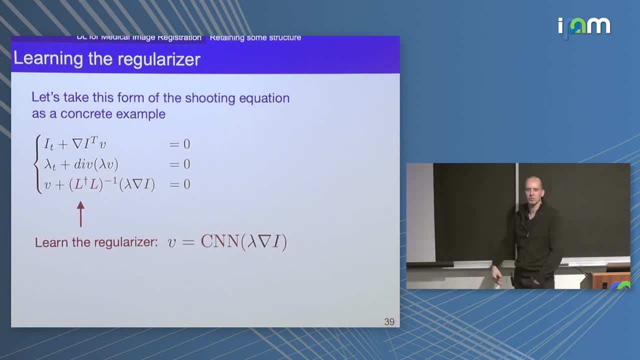 So far, Mostly this is done by mathematical convenience. You don't really know any better, so you pick something. But I want to learn this also from data And essentially I want to have something. for example, it takes the momentum or the image. 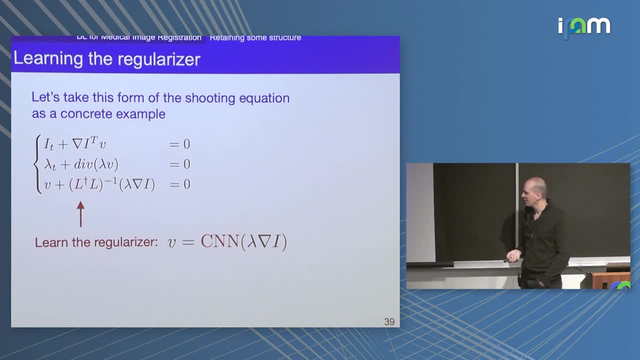 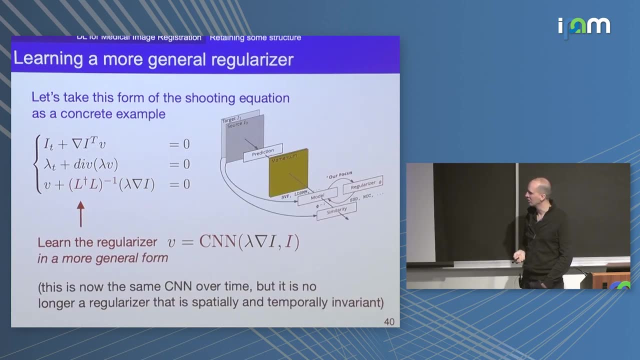 and then learns how to give me a smooth velocity field, And this raises a bunch of issues that I want to try to step here through and explain what we do here. But essentially this is what I'm driving towards, So I want to have the same model as before. 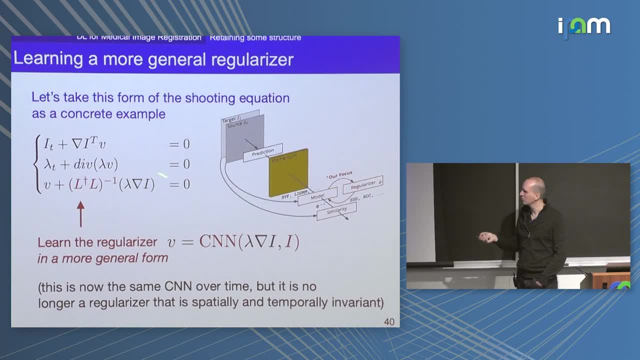 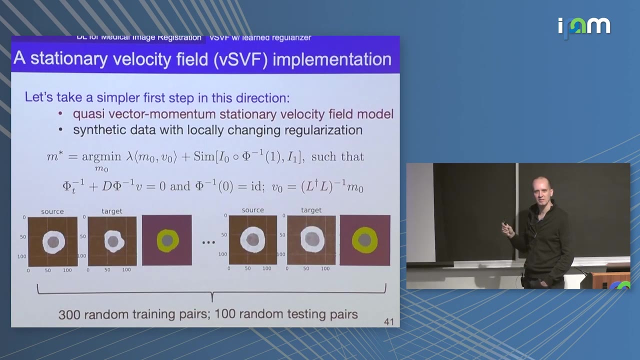 learn eventually how to predict these initial conditions, but also learn something about the regularity of what does the data support in terms of how much smoothing should they happen in different locations, and learn all of this from a big population of image pairs. So the first issue that arises here is: you can do that. 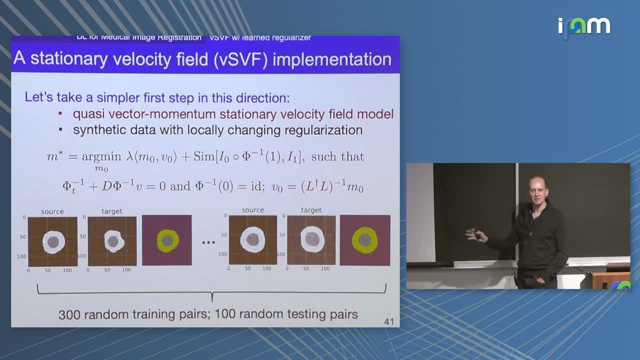 You implement it, You get some sort of result. You get excited or not, But you have no idea what you actually should be finding. So it's a little bit disconcerting. So the first thing I did, hence is I wrote some sort of simulator that 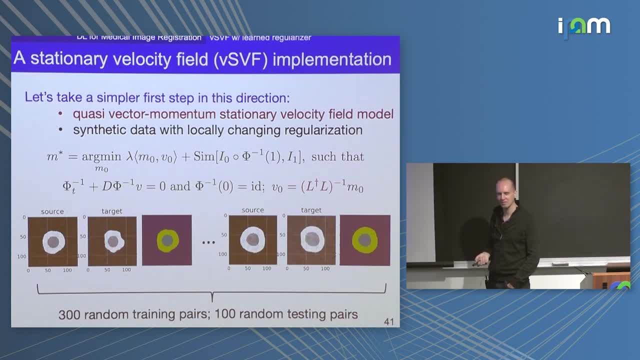 creates a lot of pairs of these artificially formed images And these images are source images, target images, And then I imposed different levels of regularity in these different regions. So basically I say this is very regular, so I smooth it a lot in this outer ring part. 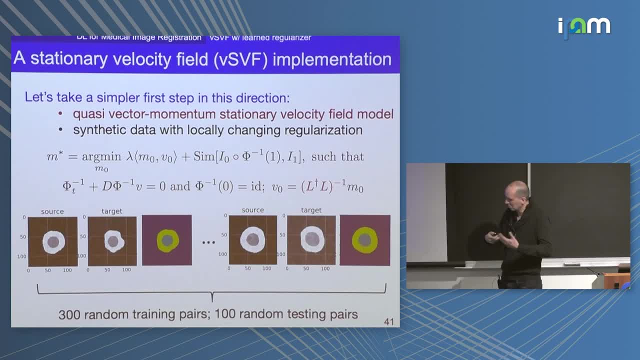 It's a little bit more permissive, so it allows to move more. And then the inner part again is a little bit stiffer. And I can, because I have a simulator, I can create a lot of pairs And I want to see, can I estimate the deformations? 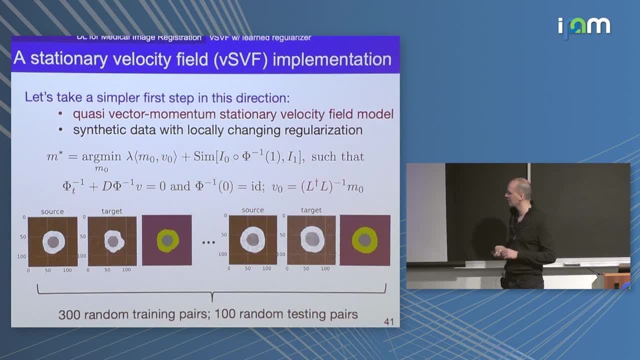 And can I estimate something about these regularity properties? And just to make the model initially simpler, I took a step back And I didn't do the full-fledged LDDMM. I essentially do a stationary velocity field where I assume the velocity field is fixed. 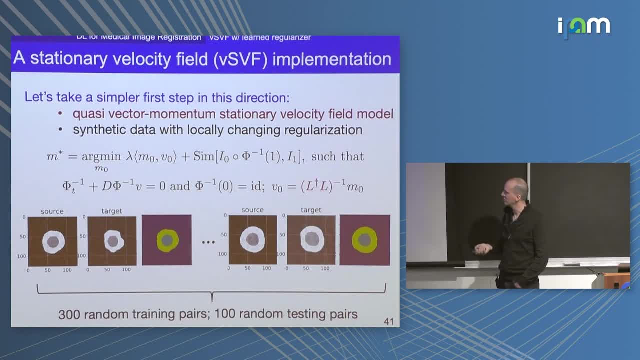 There's no equation, I'm just. I have the velocity field, I just integrate essentially this equation or the transport equation on the image. But I also penalize it in the sense that I'm predicting the momentum field or estimating the momentum field. 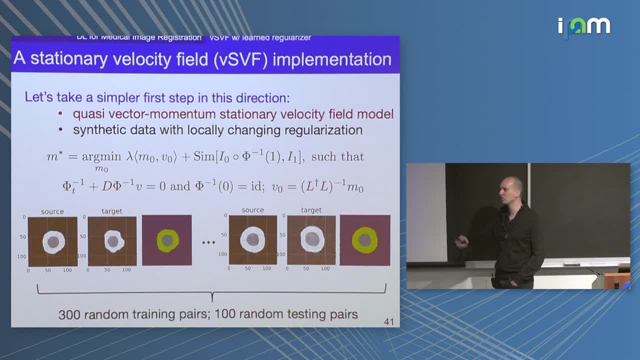 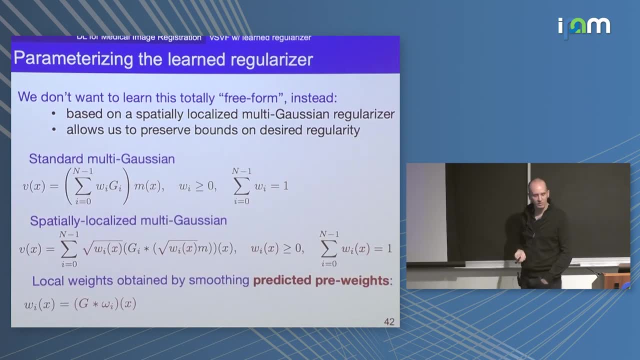 And I say I'm getting the velocity field by smoothing the momentum field, And then I want to see if I can recover some aspects of this. To be able to do this, of course, you need to define some sort of notion of how you even want to go about parametrizing this sort. 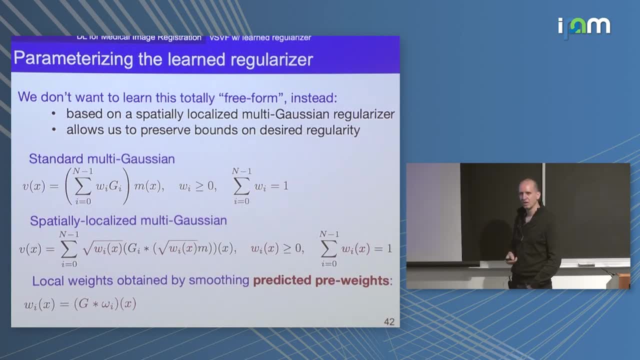 of class of smoothness that you want to consider Again, you could go about it in the sense of having a totally general neural network that predicts how the smooth velocity field should look like from the momentum. Maybe that's possible. We haven't tried this. 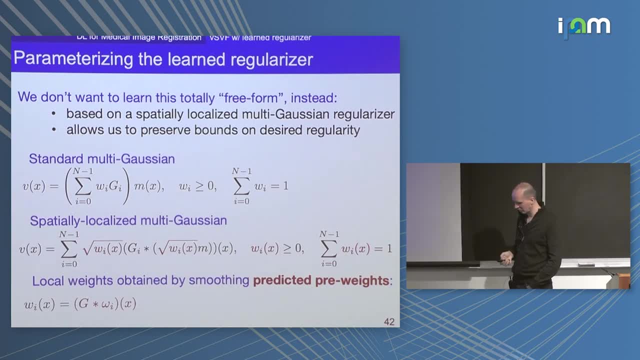 We wanted to start a little bit simpler, And the simpler thing we tried to start. we started from something called a multi-Gaussian regularizer. I think there's a convolution sign missing, But essentially you're saying you take the momentum and you get to the smooth velocity field by smoothing it. 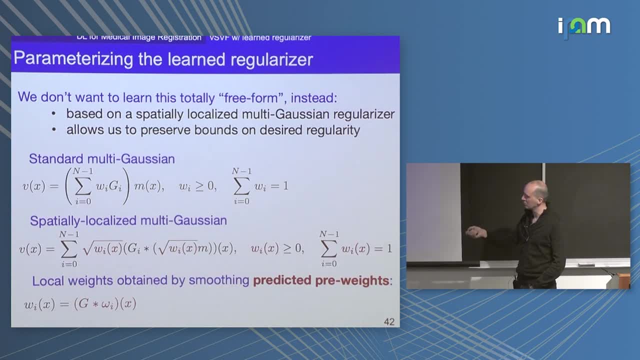 with a mixture of Gaussians, And so the mixture weights sum up to one And you have a bunch of Gaussians at different scales And you decide on the weights And then you would smooth it. So this exists, But again, this is done sort of globally. 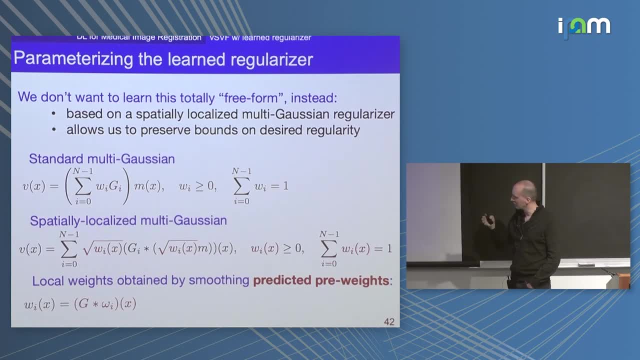 So we wanted to estimate sort of locally changing mixtures of Gaussians. So I pick a set of Gaussians And then I locally try to predict the mixture weights from which I get this. And there's a little bit going on behind the scenes. 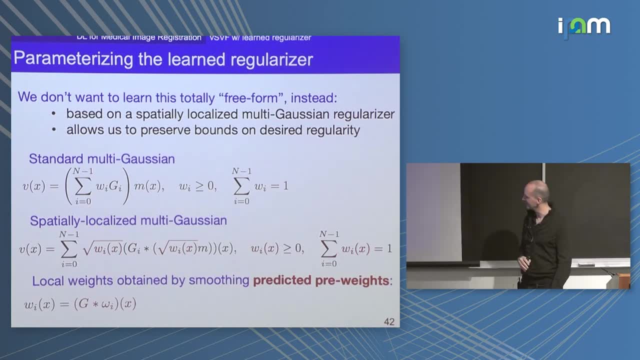 which I'm also going to put Turkish carpet over, just like I did yesterday. But essentially you could say the simplest thing is you just make them spatially dependent here. If you do this, it might be possible that it's in theory still diffeomorphic. 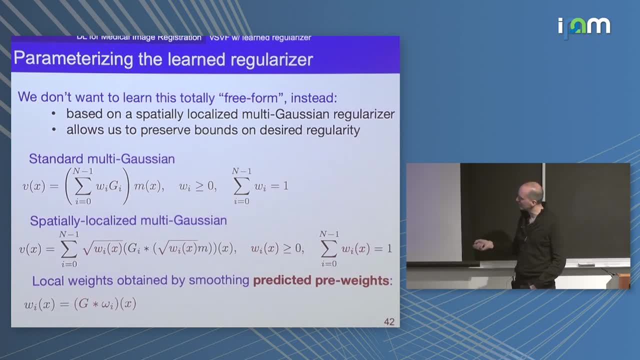 We were not able to prove it. But if you do it in this form, where you take the momentum field, multiply it by the square root of this wi of x, then smooth it and then multiply it again, then you can prove it, assuming. 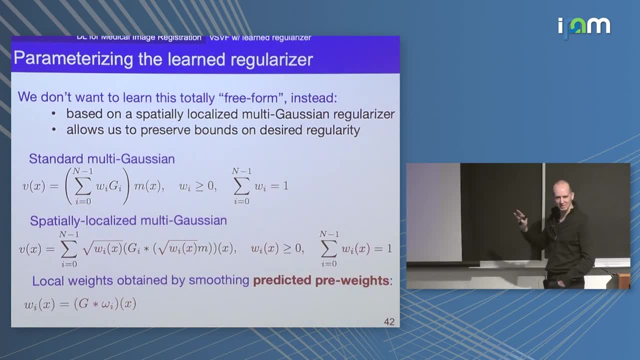 that these weights also get smoothed a little bit. So if you do this, then you can assure it. So the setup here then is really: we want to predict from the data not only the initial momentum field but also the mixture weights. And of course, if you predict the mixture weights, 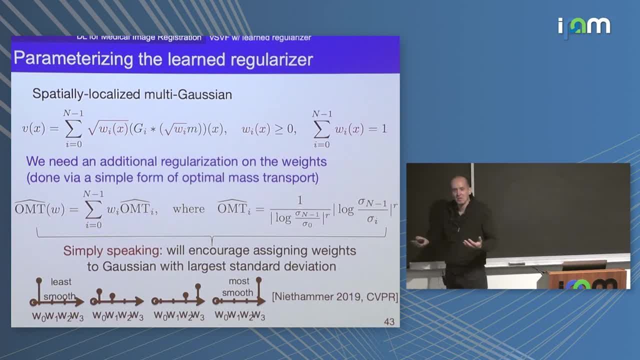 then the question is, what are good mixture weights? And again you have something that's sort of way over-parameterized with a vector field. at the beginning already, You try to take this ambiguity out of it By smoothing it, but now you introduce even more ambiguity. 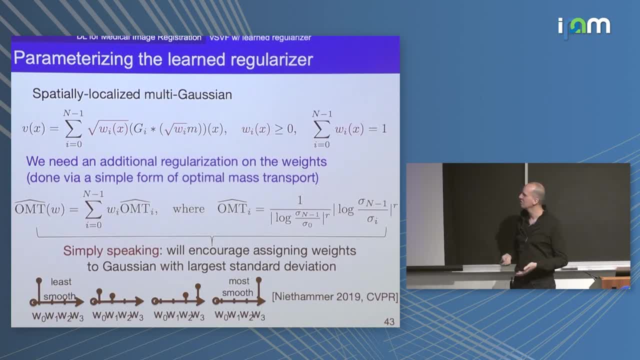 because now I have all of these mixture weights. So to get around this a little bit, I mean you can forget about this equation, At least intuitively. what we were saying is that, when in doubt, try to explain it with the simplest possible transformation. 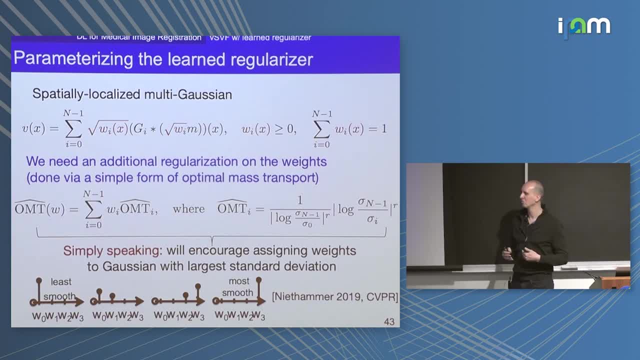 So what's the simplest possible transformation? It's probably assigning all the weights to the Gaussian with the largest standard deviation, the one that smooths us most. So what we do is essentially: let's say, if you would have four Gaussians, 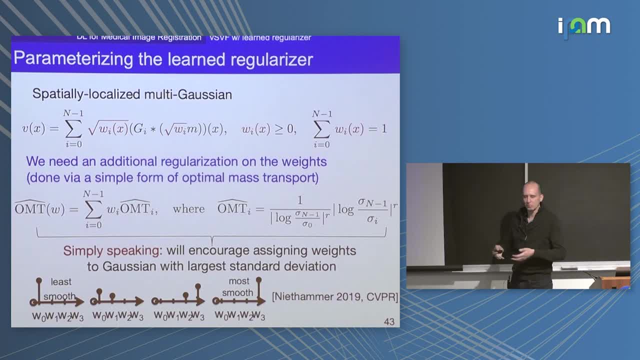 and you have weights for these Gaussians that need to sum up to one. We just regard this as a discrete distribution And then we just define some sort of optimal mass transport penalty on this. But we say: the cheapest one is the one where everything is assigned all the way to the Gaussian. 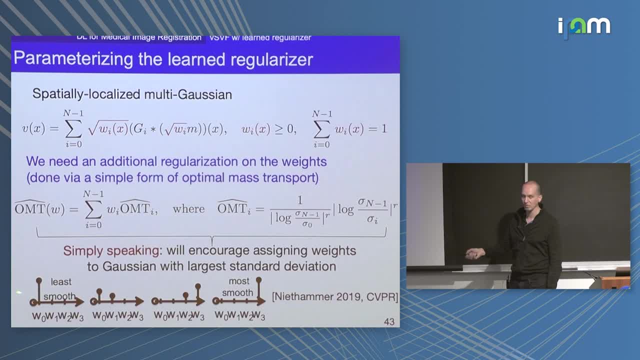 with the largest standard deviation and the most costly one is the one where everything is assigned to the one that has the smallest standard deviation, where it can do crazy deformations, And so you get penalties in the middle, And then, if you want to, you can also. 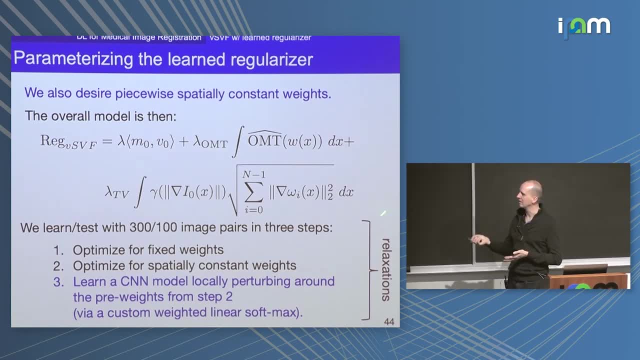 add some sort of additional terms where you say, hey, maybe you want this weight, Maybe you want these weights to be spatially uniform. You can put some total variation on it, Or you can put some other penalties if you have some sort of ideas of what you expect. 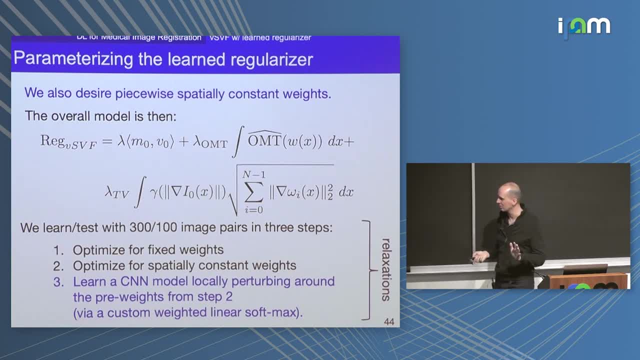 these weight distributions to be. But that's essentially the setup, And so then you can optimize for the fixed weights, Maybe you can optimize for the spatially constant weights, just to get some sort of reasonable starting point. And then you learn a CNN model like a very simple one. 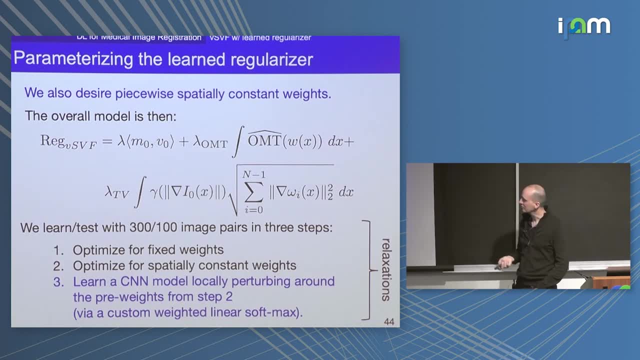 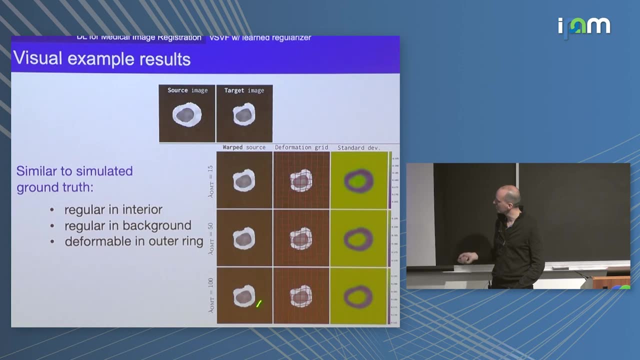 to try to predict these mixture weights. And does this work? Well, in the end it does, It does sort of work. So if you have the source and the target image here, this is the warped source. For an example, this is the deformation grid. 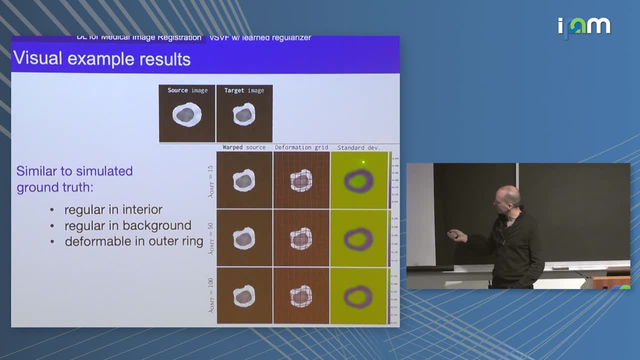 And this is sort of like the regularized estimator. So what you see here is essentially the standard deviation of the Gaussian mixture. So if it's blue it's lower, And if it's yellow it's higher. So we started out with this example. 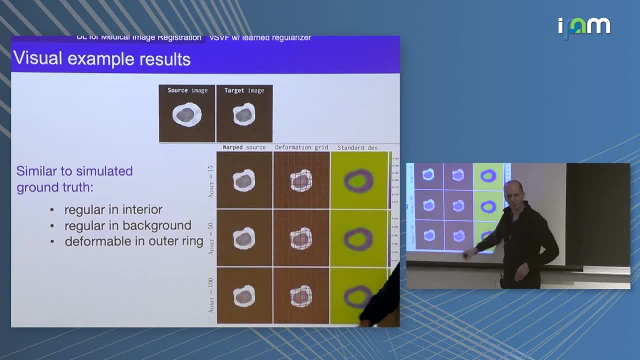 where this outer ring here is, as I said, a little bit more permissive. So the regularizer is weaker, so it can do stronger deformations, And then the outside and the inside there was stronger regularization And it may not have recovered this perfectly. 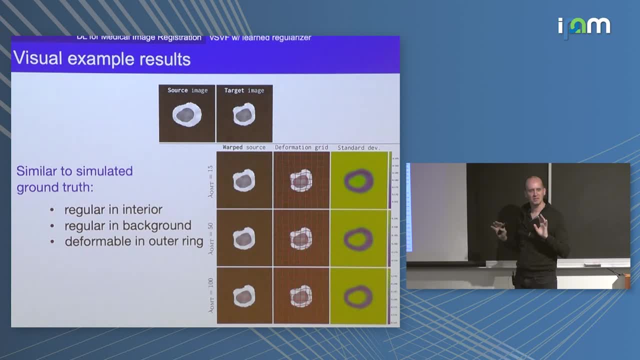 but it's sort of got the gist of it And if you feel like underwhelmed by this result, I encourage you to try this at home, because it's actually not that easy to get. I was kind of impressed that it was able to tease this out. 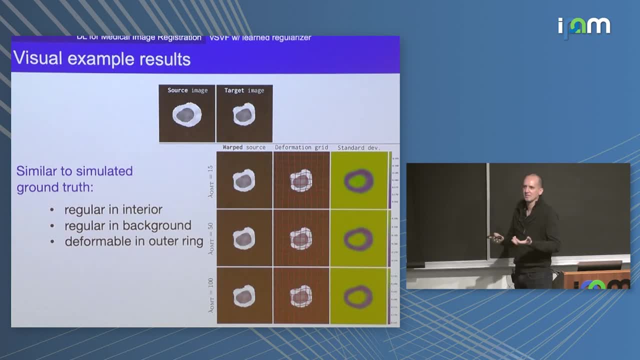 Because if you look at the deformations themselves visually, there's no real way to pick this up. I mean, you could argue: maybe- And I haven't done this experiment either- Maybe you could just take your favorite registration method and then afterwards just look at how much it locally deformed. 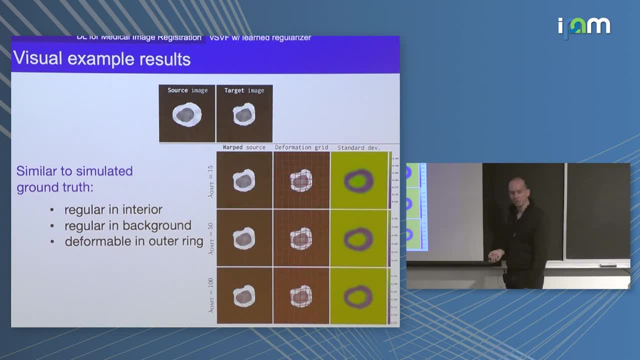 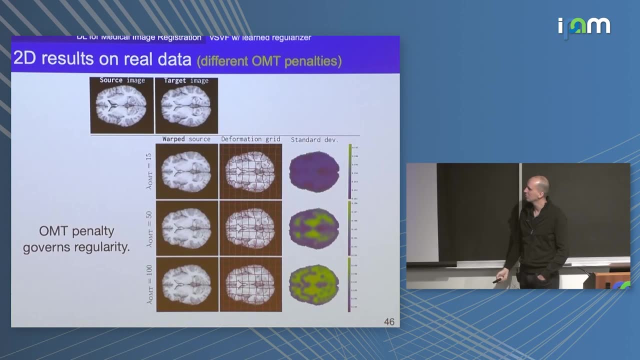 Maybe it would tease out something similar, I'm not sure, But it was able to estimate something that was consistent with what the simulation gave you, And then, if you do it in practice, you can also do this. And then the question: so these grids? 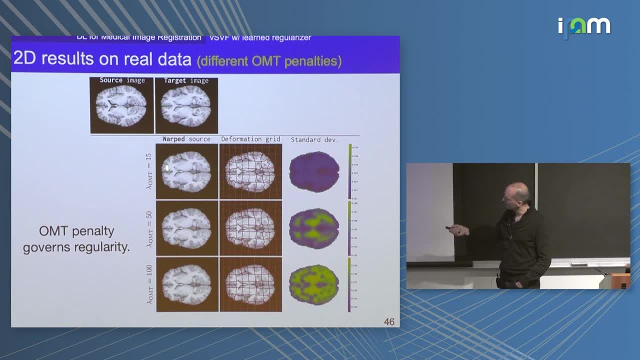 they look a little bit irregular here, But the point is that if you do this in practice, you recover some sort of structure that might have useful information. We haven't really pushed this very far yet, But it is the case that it identifies certain regions that seem to have more evidence. 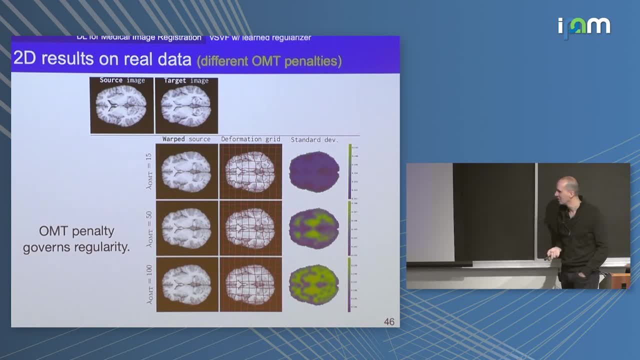 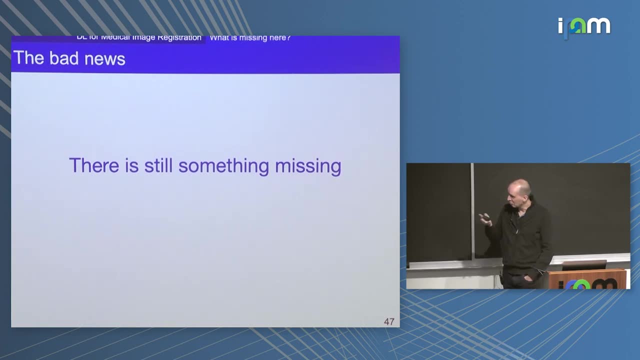 for irregularity than others. I think I'm just going to leave this here. So what is still missing here? Is there still something missing? I would argue from a theoretical point: yes, Because one thing that's sort of a little bit. 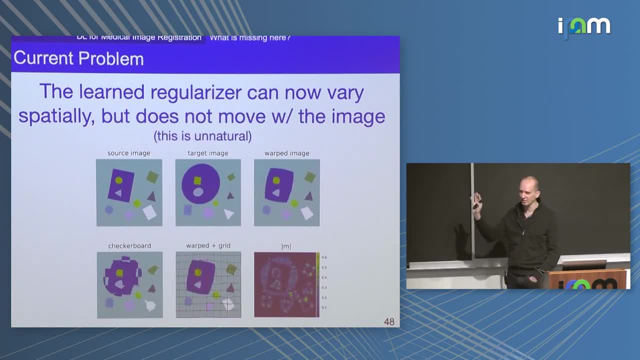 unnatural is that all these results- and maybe this also explains why the results look the way they look, All these results that I've shown you so far. they have tried to use this simpler model with this stationary velocity field, And stationary velocity field is a nice model. 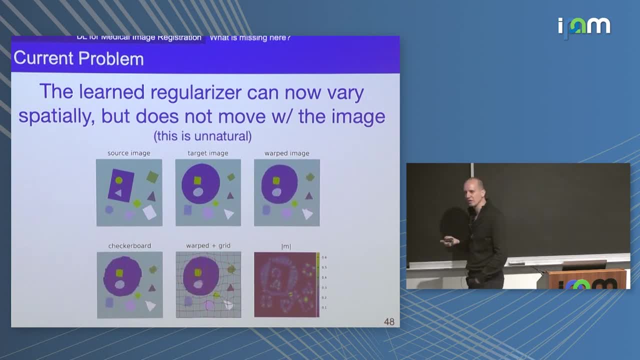 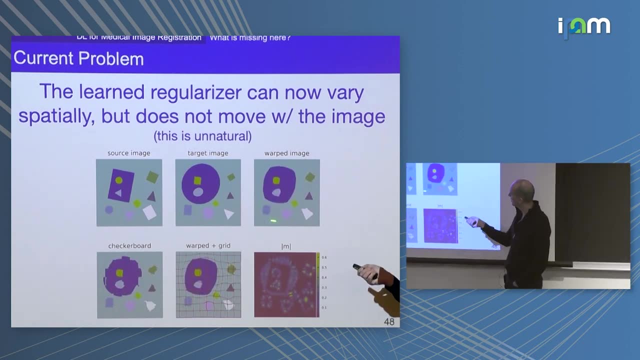 because it's relatively simple. But at the same time, if you have large deformations, it's somewhat unnatural, Because here it's sort of like an illustration of a source target image- toy example- And here you see how it's deformed. 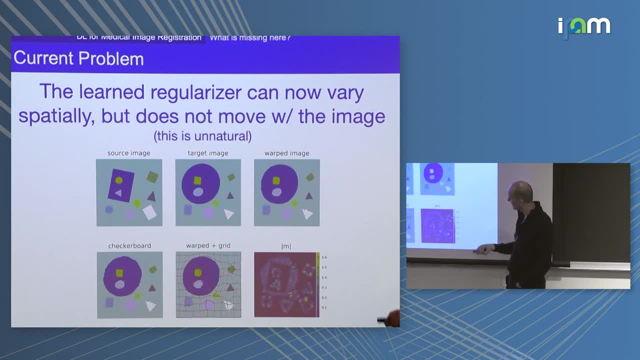 and how the grid deforms. But the parameterization is really some sort of step And you can see that the static momentum field or velocity field doesn't change. So if you have something that sort of keeps moving, in a sense this parameterization is fixed. 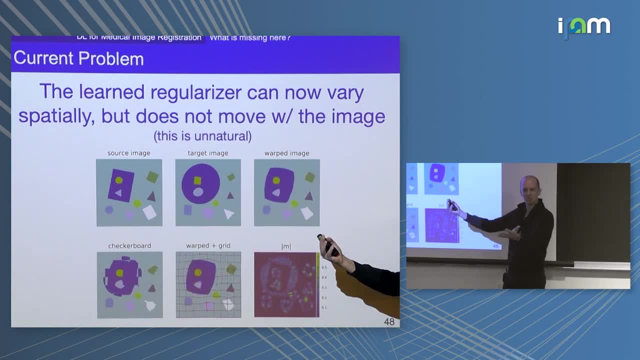 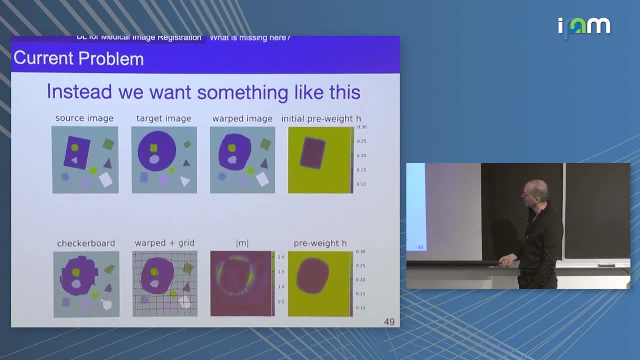 and somehow needs to explain this. It gets a little bit washed out because it cannot really move with the object. So if you compare this to something like LDDMM, this is actually not standard LDDMM. This is something we call RDDMM, because you 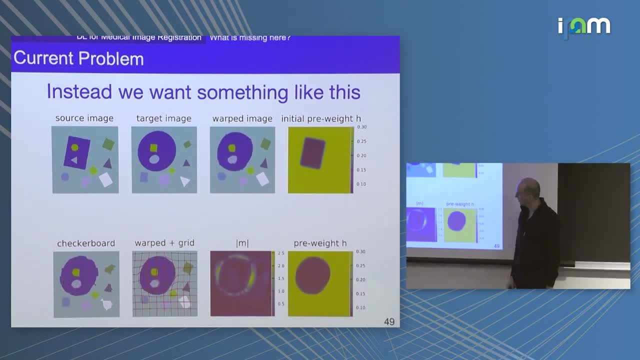 see sort of how the regularity also moves with the deforming object. But what you should note here is that this momentum sort of moves with the deforming object And in a sense it's much sharper from the model point of view. So what's missing then for us, and what? 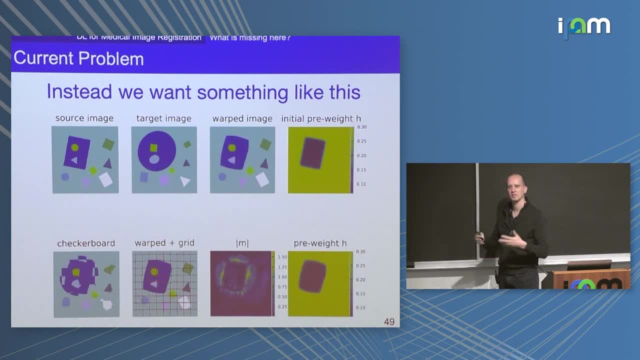 we worked on for a little bit is we try to see if you can have these sort of LDDMM-like models with regularizers that you estimate and that may change spatially, But then also that the regularizer itself moves, it deforms. 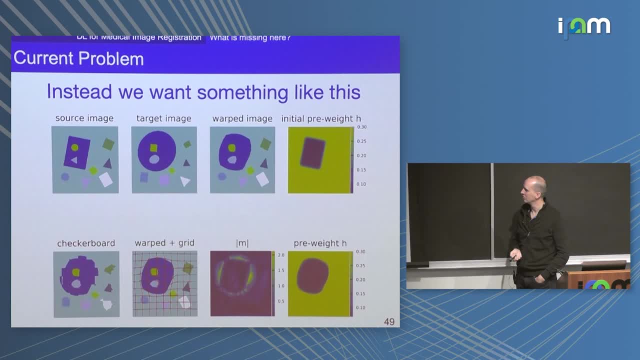 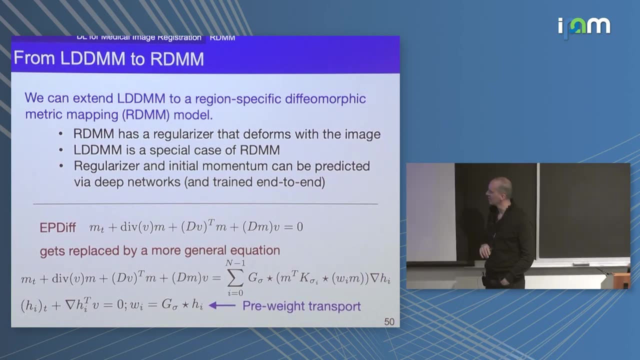 So this pushes it a little bit farther from the original model. I don't really want to belabor the point here that much. I mean, if you want to, you can look at the paper And we have the derivation in there. But it's sort of interesting to see. 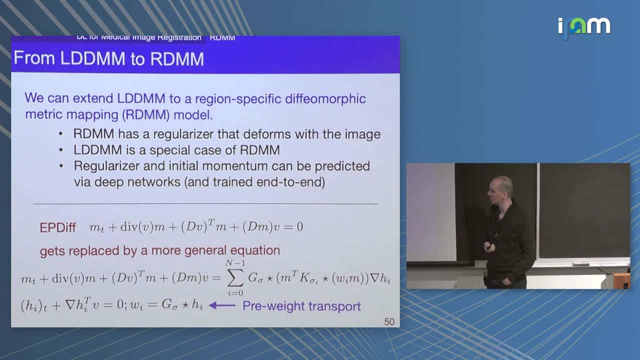 what this does to the model when you do the derivation. Remember this LDDMM model was all given by this EPDiff but it's all a Po-Carré equation for diffeomorphism. So that means the whole spatial transformation is essentially described by the initial condition. 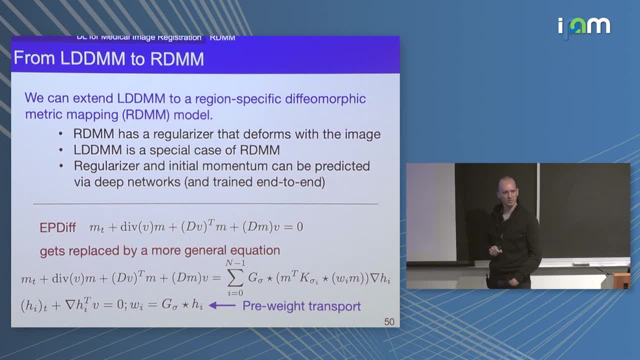 of this momentum field M, And you solve this partial differential equation. Now, when you go to this more general formulation where you say you have a regularizer that changes in space and the regularizer moves with the image because something moves and you sort of want to track this, 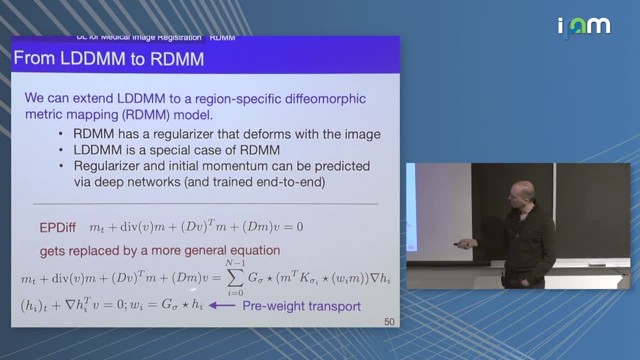 then the equation changes, But it changes in a way where the whole left-hand side remains And you get some sort of weird right-hand side. It has to do with how much you smooth these weights just to make sure they're not too irregular. 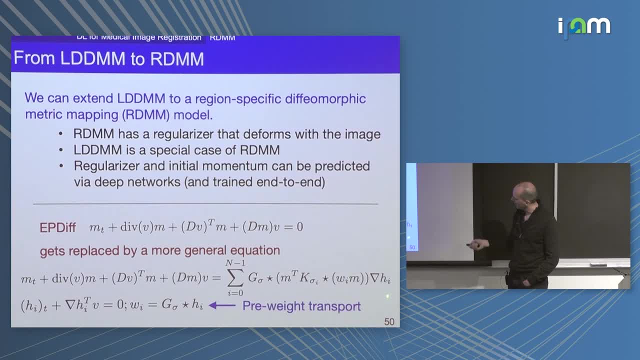 There's the smoothing itself of this momentum And then this gradient, HI, HI, are these pre-weights? so essentially, these weights that are smoothed a little bit? So you see, then, if you would have weights that are constant in space, this term would drop out. 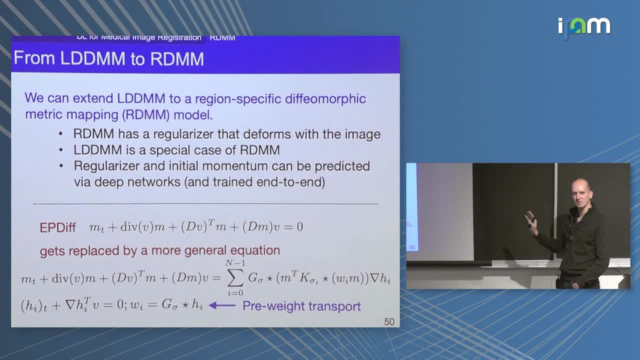 and you're back to the original EPDiff equation. So I think I'm going way too fast over this equation and I don't really want you to follow the details here. But the point is you can derive a model that's sort of like a generalization of this LDDMM model that has LDDMM. 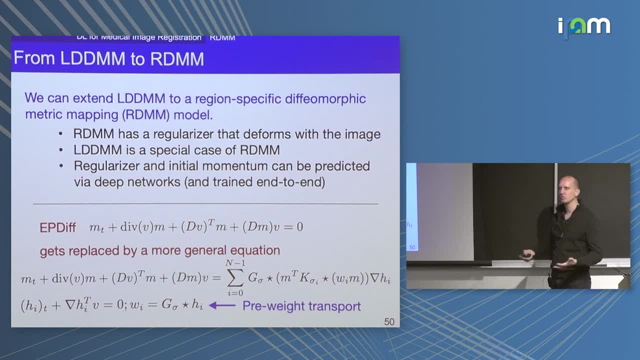 and this Euler Pocahontas equation as a special case, And it allows you to have regularizers that can vary spatially and that move with the deforming object, And if you want to, you can then put everything together- And we've also done this- where you have a model that 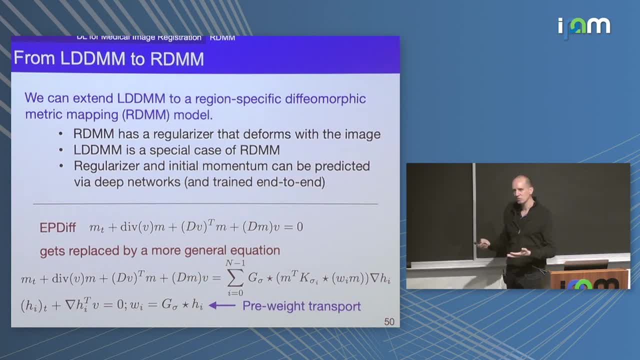 predicts then, with a deep network, the initial momentum, the weights that give you Locally the mixture weights of this multi-Gaussian is also predicted, And then it integrates out this particular differential equation and it backprops through the entire thing. So then in the end you have your favorite similarity. 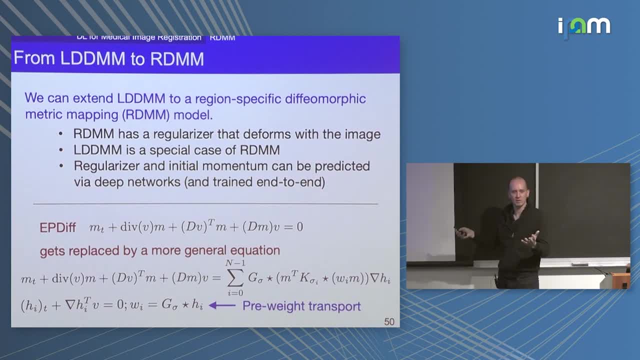 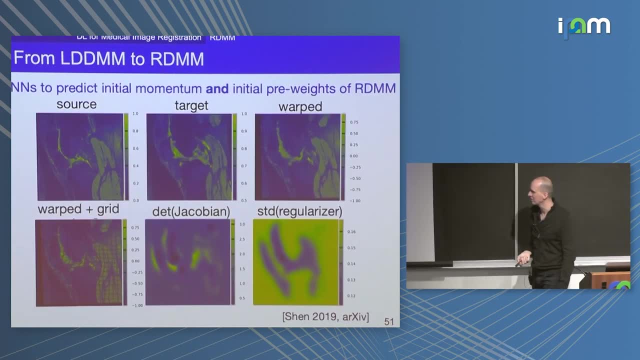 measure. It could be just based on images, could be based something on images and segmentation, whatever you want, But you can do this with this rather complex model if you want to. And here are a bunch of examples, So this was not a total variation. regularizer. 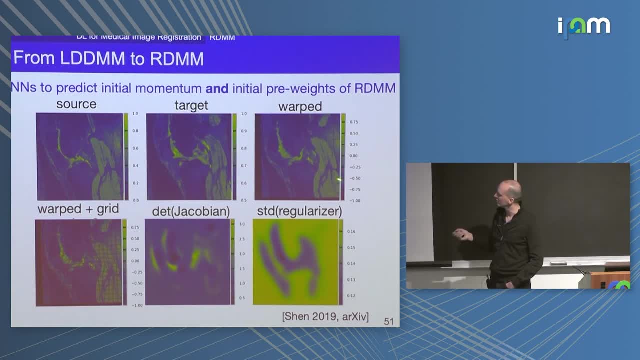 on the weight. but this is a knee image. You see a source and a target and a warped image. And then what was estimated here is that it wanted to have a little bit more freedom in terms of deforming things at these particular locations of the knee. 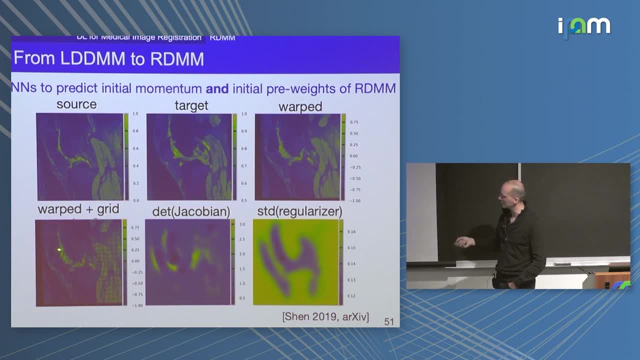 And I think this sort of makes sense. I mean, probably there's more variability that you see sort of at these interfaces of the bone than on the inside of these bones and then also on the outside. So I'm not sure exactly what the best use. 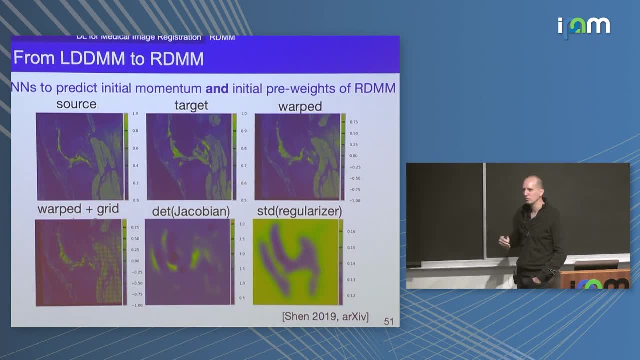 case for this methodology is. But I find it sort of interesting that when you take this more population point of view and you estimate something over large sets of images, you can tease out information that has to do with how much regularity the data seems to support, based on the model that you imposed there. 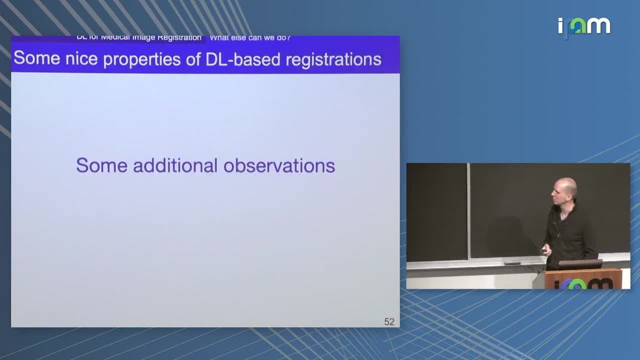 So I have a few more minutes, And in these few more minutes I'll give you a little bit of additional observations that go beyond what I've talked about in this model and maybe also a little bit more general about registration and deep learning. So the first thing is, of course, 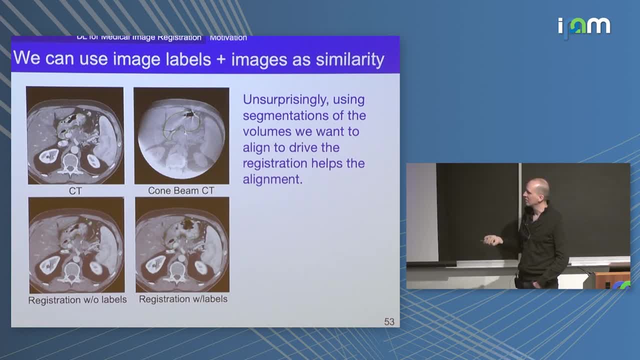 when you do any registration, with deep learning or not, if you have these very complicated registration problems. here's between CT and cone beam. CT images look very different. organs change a lot. If you drive everything just by the images it might be very complicated. 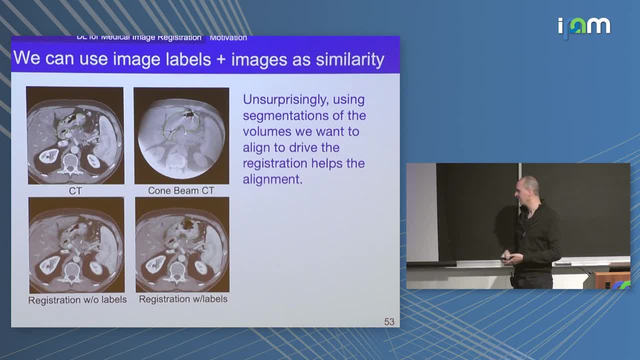 Because a standard image similarity measure like SSD or normalized cost correlation and mutual information has absolutely no idea what it should focus on. These are nice measures but they're sort of global, But there's no notion of what really matters in the image. So, in the extreme end, what you could say, 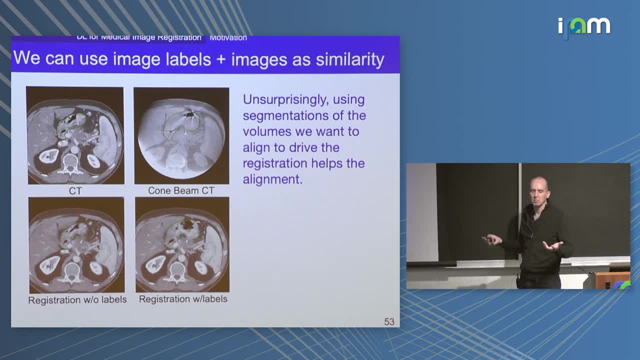 well, if you know what matters in the image and you just segment these parts, then probably, if you use the segmentation to drive the registration, you'll do a better job, And there are a bunch of papers of people that have explored this, including also. 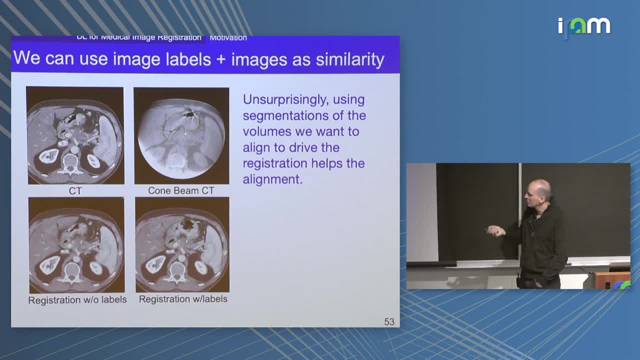 some of my students And of course even in classical registration. if you use images in segmentation, then by construction you'll probably align these models better Because you make it more problem specific. You essentially tell the registration algorithm. these are the areas I really care about. 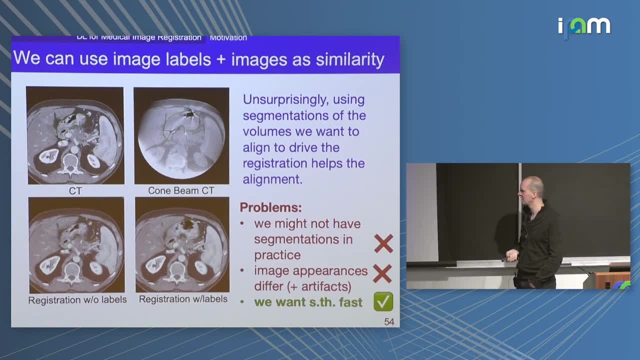 The problem is that in practice you're not going to be able to do that, So you might not have these segmentations for all of these images. Maybe image appearances differ, And sure you might want something fast that we can deal with with these deep networks. 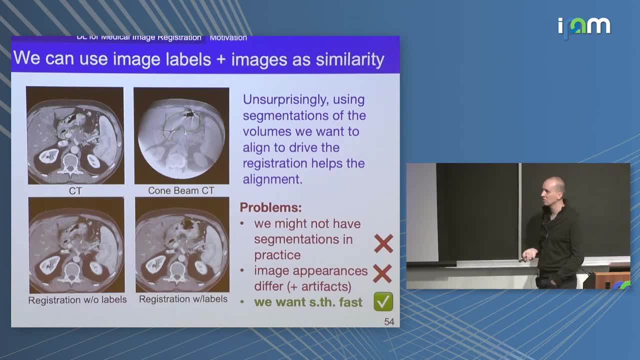 But the nice thing is that also not having segmentations at test times is something that you can do with these deep networks, Because these deep networks can learn things that they see during training And then you might not need it at test time, And I think this is really without going too much. 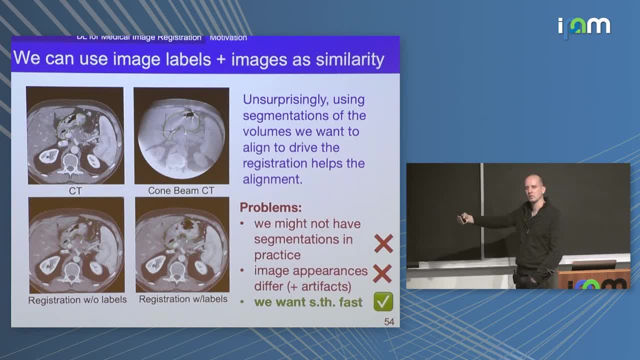 into detail here. This is one of the benefits of doing this with these machine learning approaches Because, opposed to these classical registration approaches where you have two images and then maybe two images with segmentations when you learn it over an entire population, 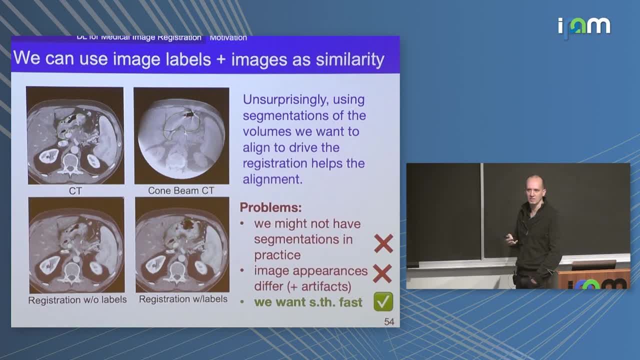 there may be some data that's available during training, but not necessarily at testing, But it can somehow give you a model of deformation that's a little bit more reasonable and can help you to learn good transformation models. As a case in point, the very first paper we've actually 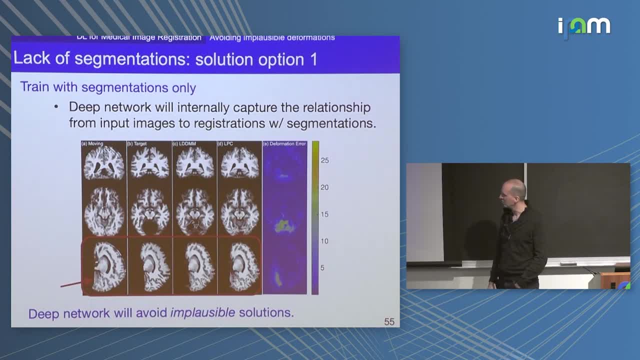 version of the very first paper we've done on this in 2017, we were sort of curious to compare how the performance of this deep network was in comparison to just straight up numerical optimization, And we did this on one of these standard registration brain. 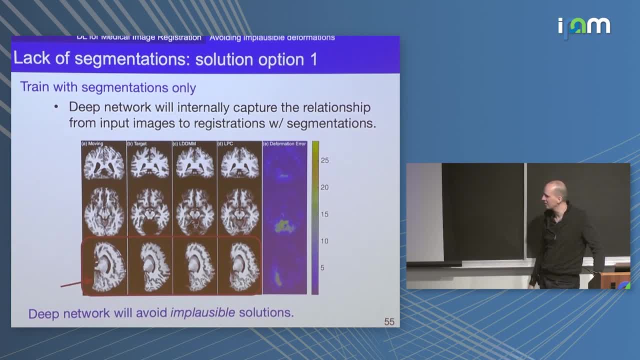 image data sets that are out there. I mean they're all relatively small but they're standard. So we compared against those And it turned out that for some of these images it seemed to do a horrible job. It seemed to be very different. 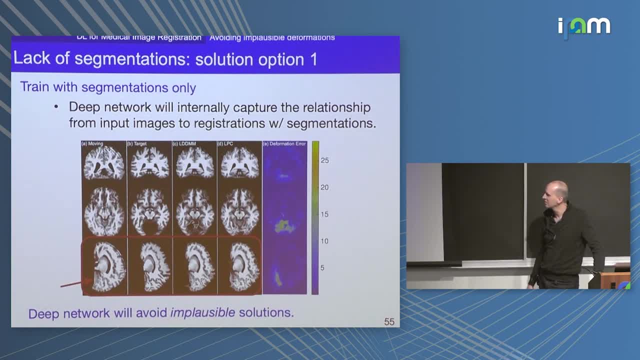 And so we looked at it. We looked at these images, and it turns out that one of the reasons why it was so different is that these images they had sort of like a poor version of brain extraction, So the brain extraction didn't work very well. 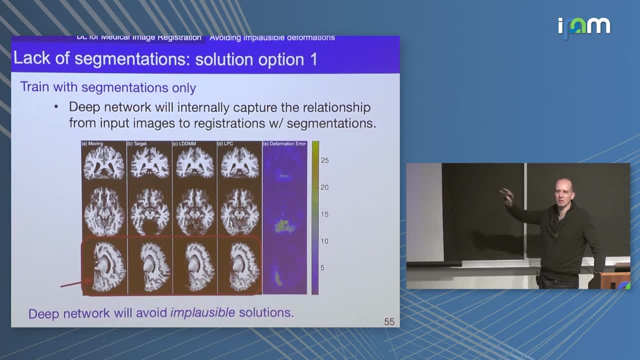 So if you then do registration between a brain image that has been extracted well and another one that's not that extracted well, if you do this with your favorite optimization approach, that method doesn't really know that this is the case, So we'll just go for it. 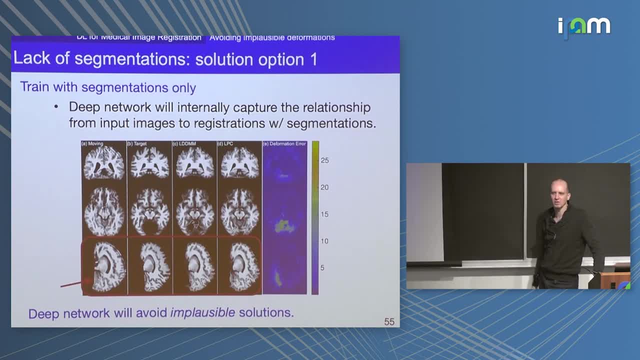 We'll push as hard as possible, We'll make this transformation, And it might not be realistic. And if you do this, it's not realistic. And if you do this with a deep network, what happens is that, behind the scenes, if you want to or not, 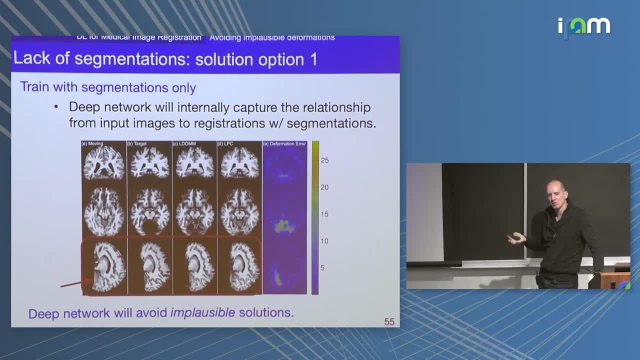 it's going to learn some sort of essentially statistical model of what the deformation space is, And this can be good in the sense that it might avoid doing transformations it has never seen, So in that sense it's not going to push like crazy trying. 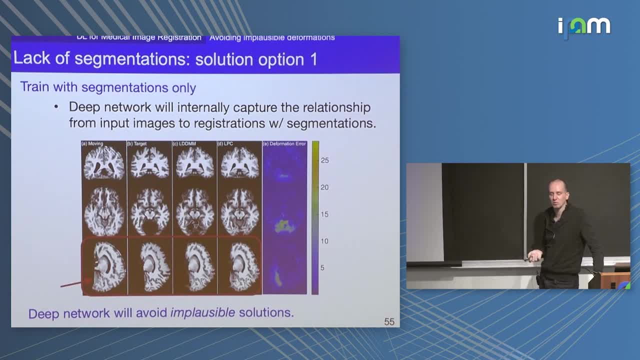 to align structures that are not supposed to correspond because they're different in these two images. But of course, this can also potentially be a bad thing, because if there would be some case that you want to capture and has not been in your data, it 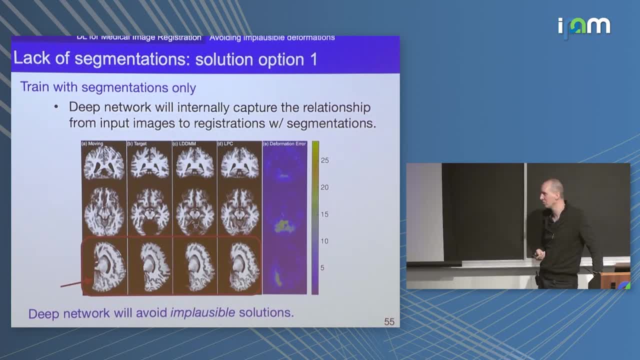 might refuse to do that as well. So I think this is just sort of like a high-level comment, in the sense that it has a nice behavior, in the sense that it captures somehow the space of deformations that it has seen And it uses them to construct a new transformation. 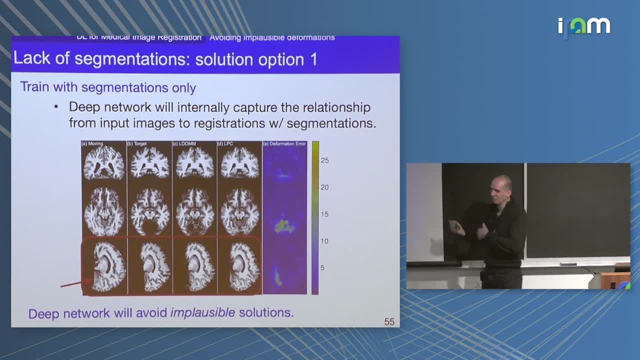 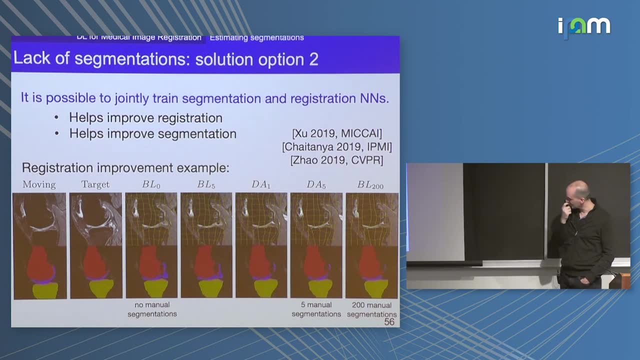 when it predicts. But the question is: do you like to be nice, Right? In some cases, maybe you don't want this property. What I also wanted to say is, as I said earlier, if you use a standard similarity measure, 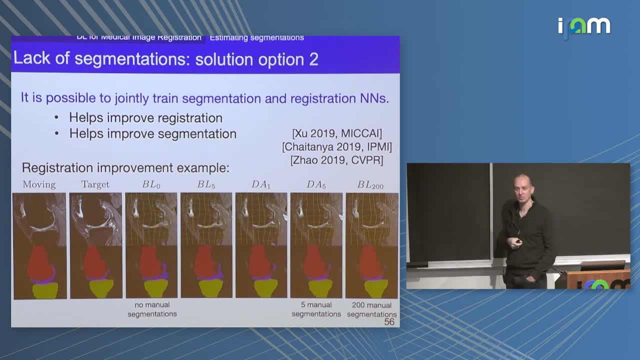 then oftentimes you don't really know what the registration should focus on. So if you drive it with additional segmentations, you could potentially do much better. But if you sort of combine registration and segmentation, these things can reinforce each other. We've done some work on this at McKay last year. 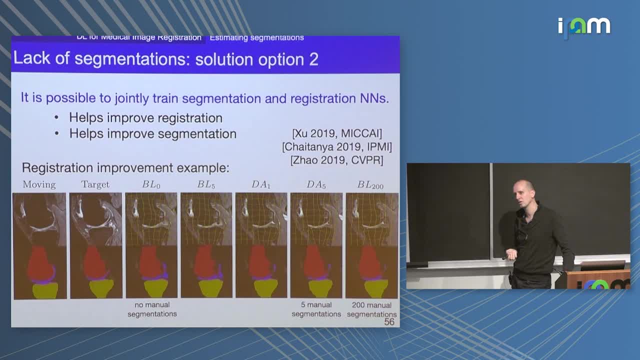 where we tried to jointly train a segmentation And the registration network. Ender has some work. It did me, I think Ben had something at McKay And then I think one of Adrian Dalcha's students also had some work. They essentially all go a little bit in the direction. 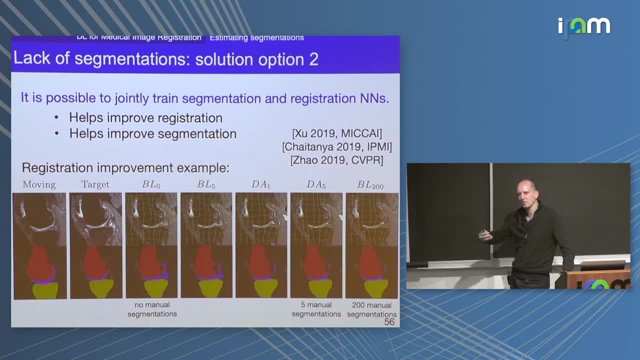 if you wish, that it uses registrations of, potentially, images that are unlabeled to give you some form of intelligent data augmentation, if you want to call it like that. And here, in this particular case, again, this is an image of the knee. 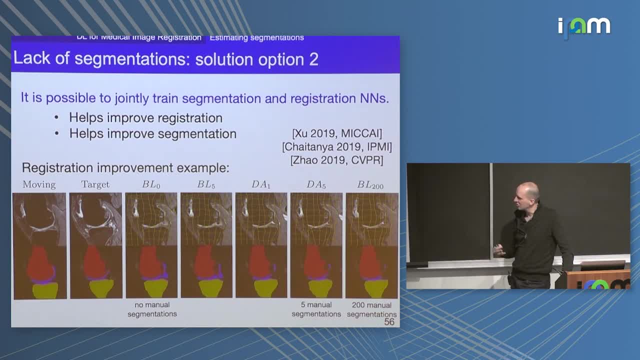 And if you're interested- it's sort of like in registering- right, You're in the cartilage. If you just drive this based on the images and if you don't have a whole lot of images to train on, then in some cases you might do a very poor job. 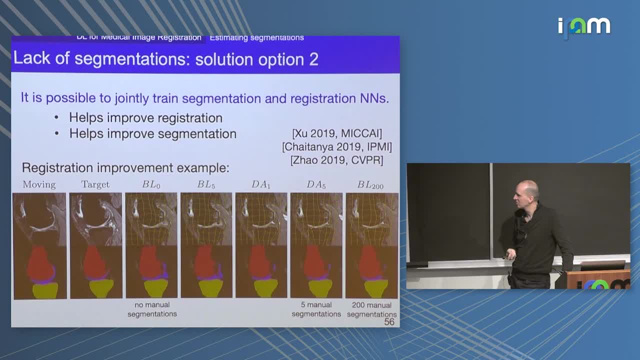 But if you jointly train a segmentation and registration network, you can get away with very few images for training. So what these images here show is: this is an example where you just train the registration network And it uses the image and then labels for 200 images. 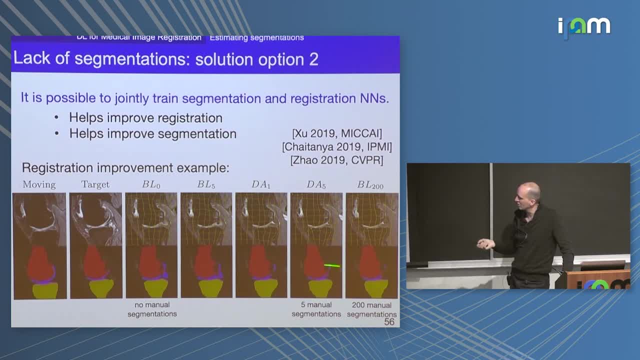 And you do a pretty decent job at doing this registration. It looks good after registration. If you just do this with five, just directly the registration, or just with five images, you get sort of these really weird deformations because it couldn't properly learn this. 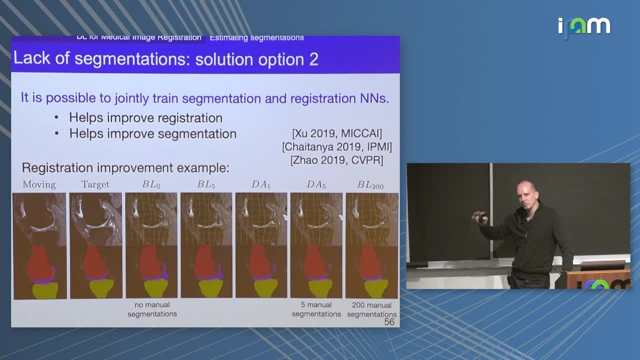 But if you do it in a way where you have the registration network, learn from unlabeled images how you essentially augment the data you can with very, very few images like five or 10, learn a pretty decent segmentation network And then the segmentation network can drive the registration. 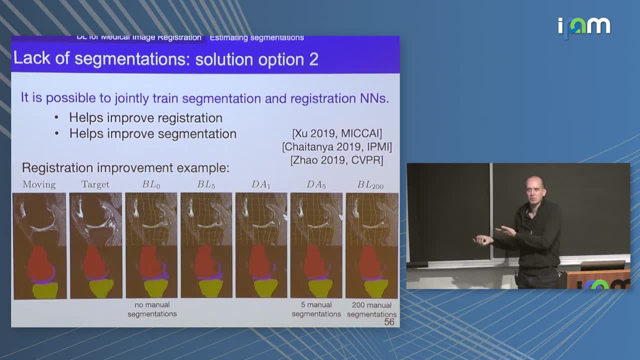 Then it can sort of mutually reinforce itself And you can do much better for these thin structures. in this particular case, And I think for me, combining deep learning with these types of models, I think these are the more exciting directions because if you just take your plain old loss, 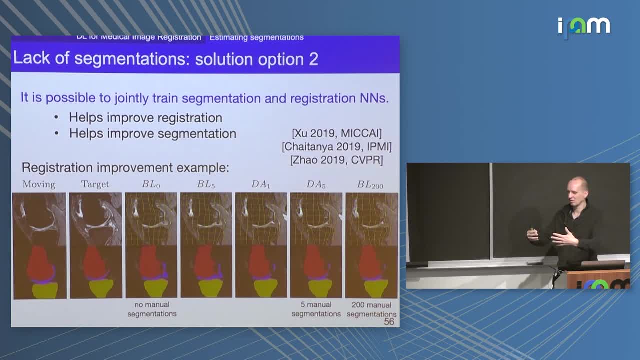 function and you make it faster by putting a deep network in front of it, which we have done. so I'm criticizing myself, But this is sort of like gives you something faster but not necessarily better, But if you push it towards creating some sort of additional information, 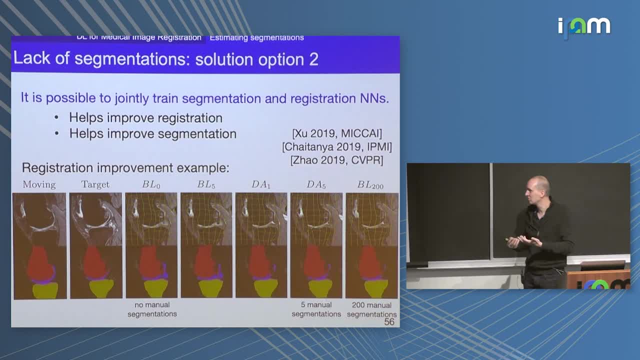 that you traditionally may not have. then I think there's hope that you can outperform some of these more traditional methods and that they are, sort of like, more nicely behaved because they focus on the regions that you think really should matter, or the algorithm figures out. 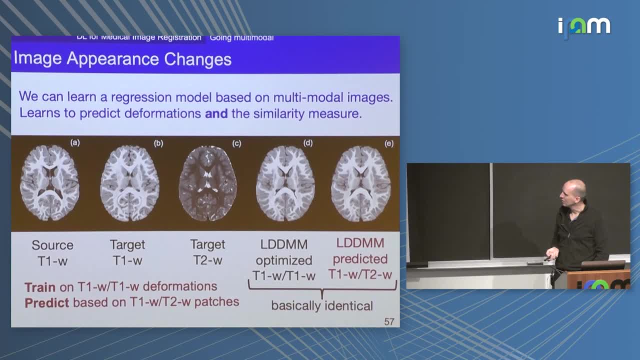 that they should matter. And then the last thing I'm going to just briefly state is that, Of course, these models, they also have the ability to learn, in a sense, more nontraditional image, similarity measures, And this can be done in different ways. 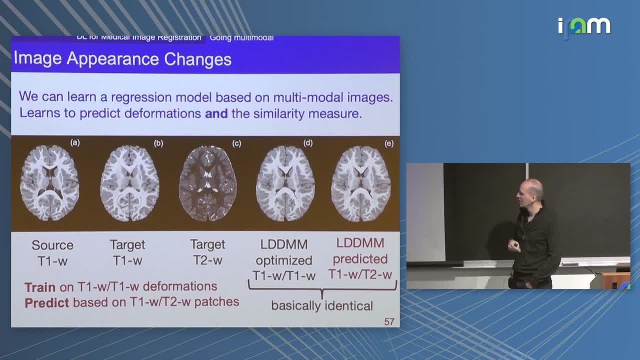 And people have proposed different ways of doing this, Some of them also with like GANs or doing some sort of features that are somehow deeper in the neural network, But from the most primitive way of doing this. here's an example result of where we just had a set.